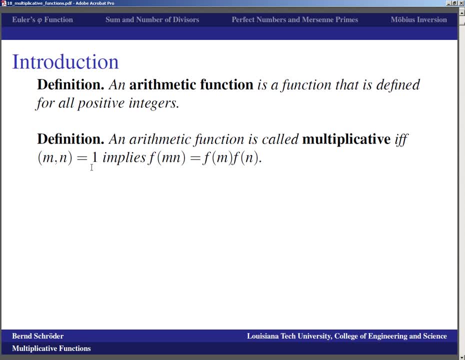 that the greatest common divisors are. The divisor of the two factors is 1. We have that the value of the function at the product is equal to the product of the values of the function. A function is called completely multiplicative if, and only if, we have this property for all m and n. So if, for all m and n, we have that f of m? n is: 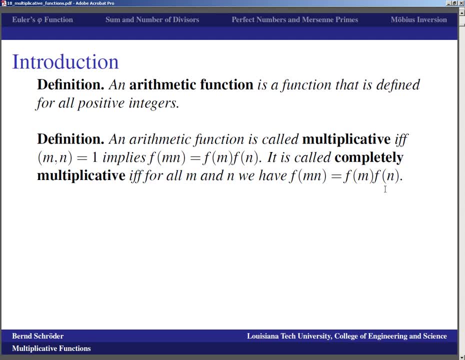 equal to f of m times f of n. That is substantially more rare to occur and we're not going to see it very often here. So in this presentation we will see that Euler's phi function is multiplicative. That's that section. We will consider the sum and number of divisor functions. 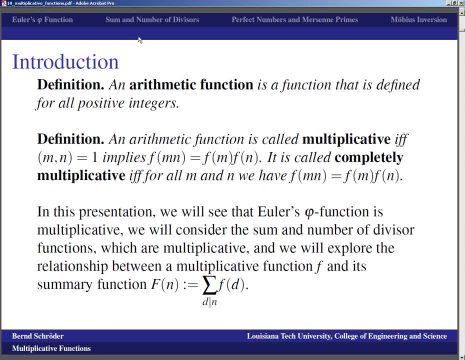 which both are multiplicative. That's why they're in this presentation And we will explore the relationship between a multiplicative function, f, and its summary function, which is capital, F of n being the sum, over all divisors of n, of the value of the function. 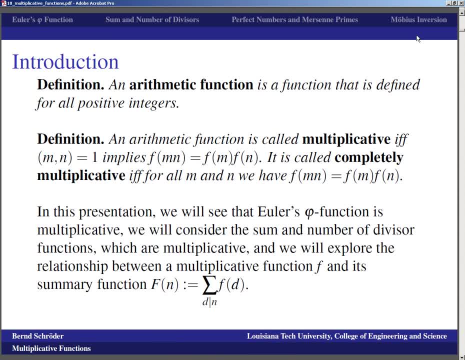 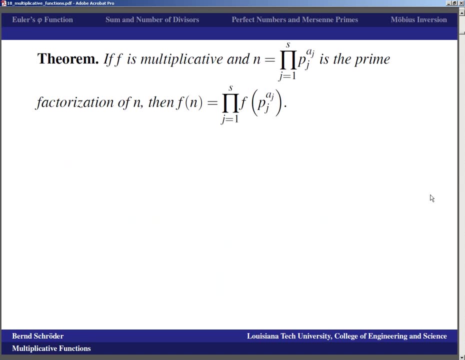 lowercase f at the divisor d And that ultimately connects to Moebius inversion and perfect numbers and Mersenne prime numbers. The problem here is that there are some where in between there They're a notion that is better investigated using multiplicative functions. Okay, so first quick little theorem: if the function 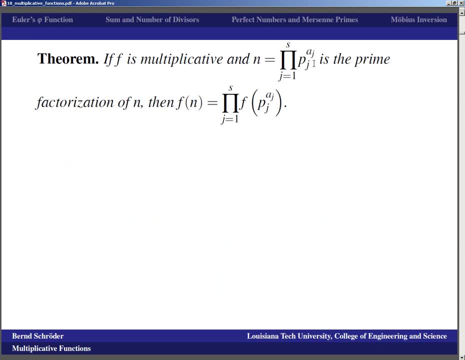 is multiplicative, and if the prime factorization is the product P j to the AJ of four m, well then f of n is just the product of the F of PG to the aj, And that ought to make sense, because 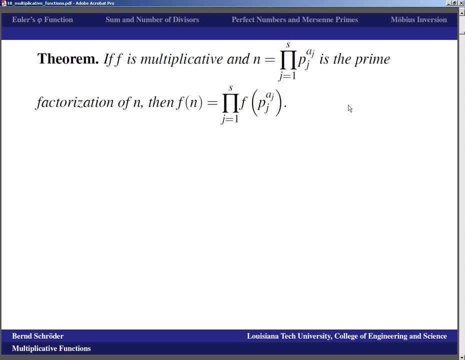 after all, the divisor one. so the product should move out, and the proof is, in fact, a quick induction on the number of factors. uh, the base step for a since trivia, look at the trip. is that not, then, or then, the base step? well, i don't think that's too crucial right now. 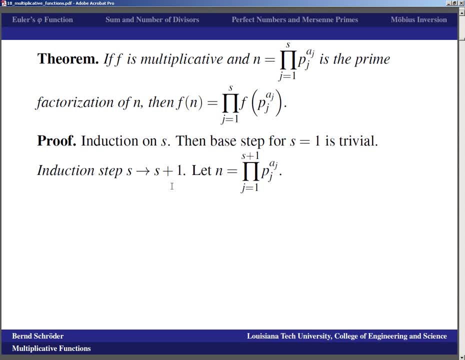 uh, the induction step from instead to s plus one is that we did in the i have a private actor, as they should, with this plus one factors. well then, if often is if of prime factorization, we can split off the last factor, so this is f off product of the first s factors. 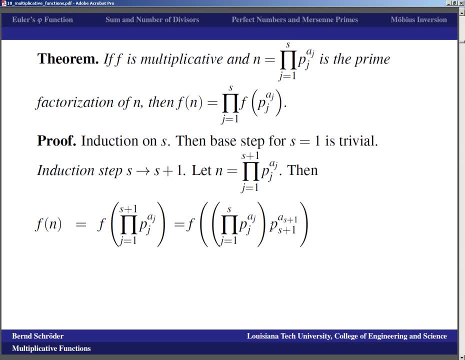 times the last factor in, because the prime number p s plus one, is different from all the other pj. we have to take a discredit by two years one, and so that means that this is if off product of the first is prime factors. uh, with their powers. 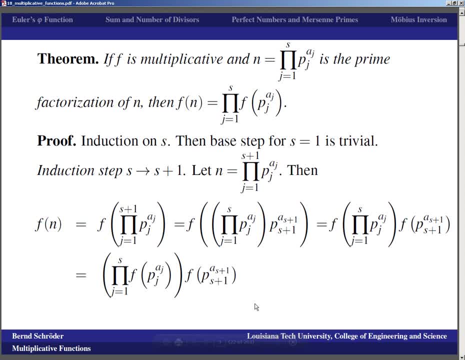 times. if of p s plus one, two a s plus one, then of course we use the induction hypothesis because we can pull the function into the shorter product and that means that effort and there is the product: g equals one, g s plus one at fourth pt to the a, j, as is. 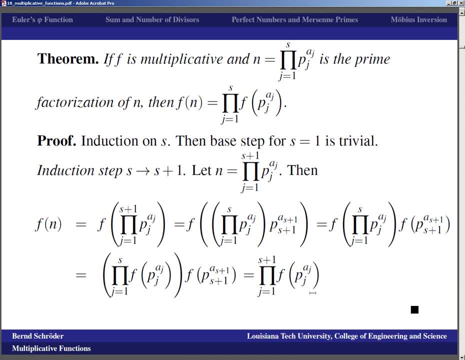 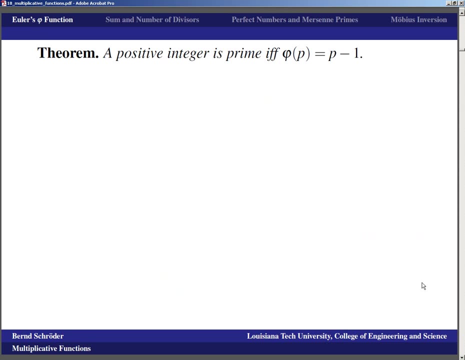 and uh, that's already. one of the nice things about multiplicative functions is that once we know what these functions do, when powers of prime numbers, we pretty much what? no, put those functions to overall as long as we can talk to the. so now uh, 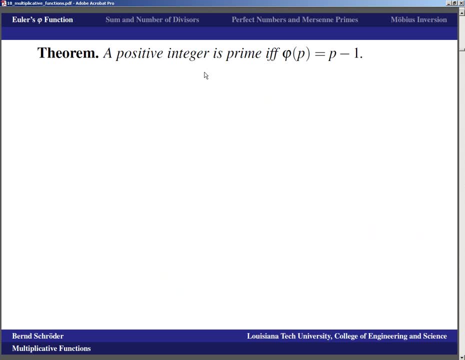 in quik view and that connects to the. the function, and that is that it's a, a positive integer, is a prime number if, and only if, field psp months, when that shouldn't be too bad because, after all, uh, the fee function gives us the number of all numbers smaller than p that are relatively 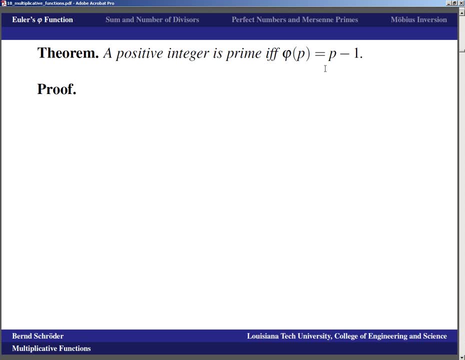 prime with the. so that sounds like it ought to be the right thing and it shouldn't be too hard left to right. suppose our, for our number is prime, with p is primed in for every number between one and p minus one. we have that the greatest common divisor of the number in p is one. 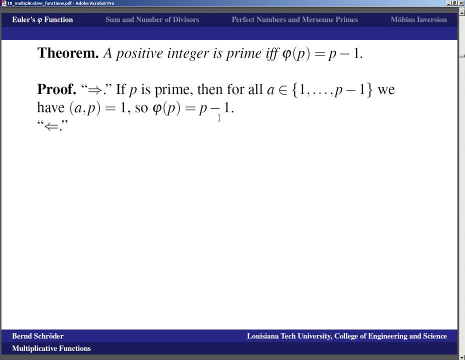 and that means field p is people. the other direction should be similarly easy. if field psp minus one, well, that means that the greatest common divisor of a mp is one for all integers, from one to p minus one. and that means that he is trying because it doesn't have any divisors strictly. 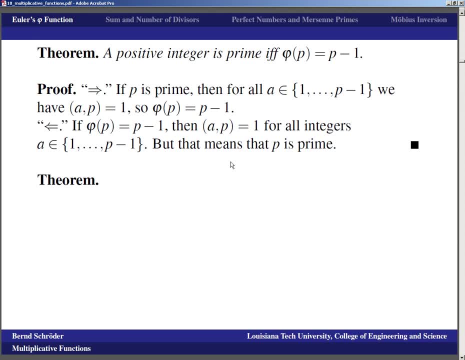 smaller than p, except- and that's it for that one next year, and is about the order fee function at that power of the prime number, so that pb a prime number in a positive integer, then field p to the a is p to the a minus p to the a minus one. 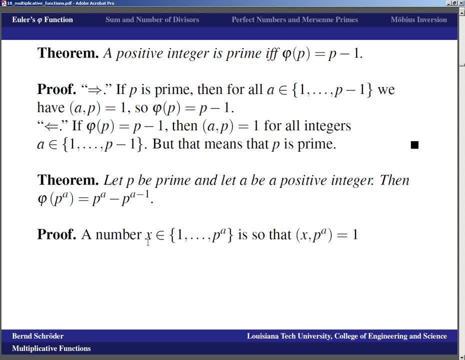 into proof is accounting argument mainly, and number that use between one and p minus one. p to the a, minus one could also go with p to the a, because we're talking about greatest common divisor with between the number in p to the a p one. well, that's the case if, and only if, x is not pro. 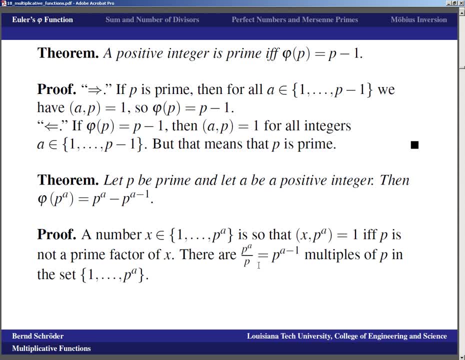 if he is not a prime factor of x. well, there are p to the a over p equals p to the a minus one multiples of p in the set one through p to the a. so we really want to focus on p to the a. but the statements 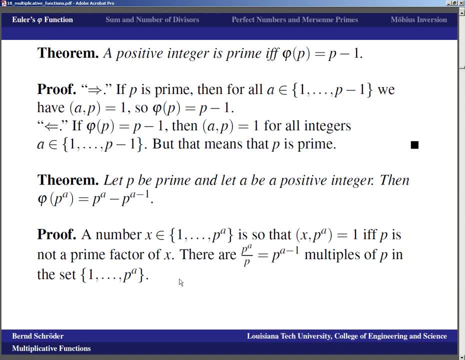 remain true. and uh, well, that means, of course, these are the numbers in the set went to p to the a. p to the a is one of them. these are the numbers that would have to be excluded from the counting of numbers that are relatively prime to p to the a, and that means: 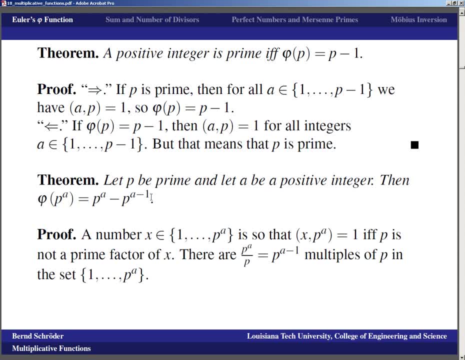 from these p to the a numbers, we have to take p to the a minus one numbers out. and we can see why we didn't want to go to p, p, p to the a minus one, because the exclusion would take p to the a out anyway in this fashion. 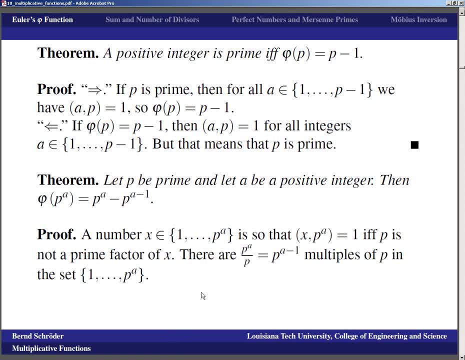 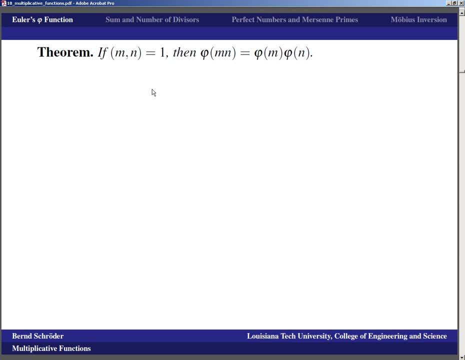 the counting is easier because we don't have to keep track of extra class ones who can what? now still talk about the fee function. yeah, here he is the fear, and that says that the fee functions not negative. so we want to prove that if we have two numbers, m and n, who was greatest common divisor as 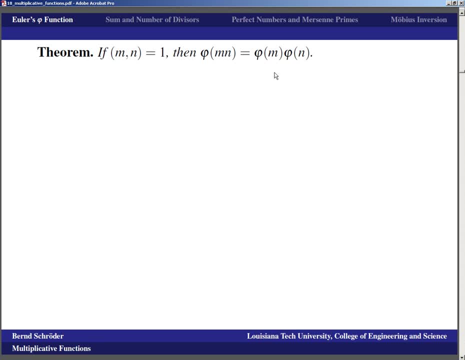 one. we want to prove that, then, field in times in its field in times in. the proof is the following: will split up the set of numbers from one through in times in and we will split it up by remainders. so the set of numbers from one through in times in. 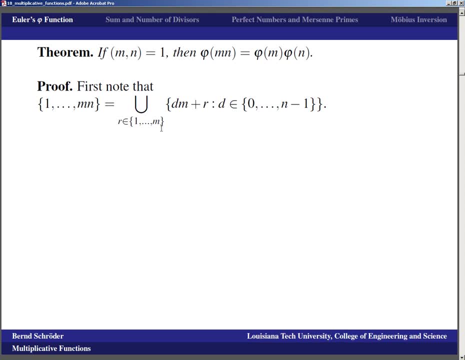 is the union overall remainders to be one in in. so we're going to you not use remainders zero, we're going to replace those with remainders in, uh, so it's a beautiful overall remainders. uh, we wanted him of numbers of the forty times in class are. 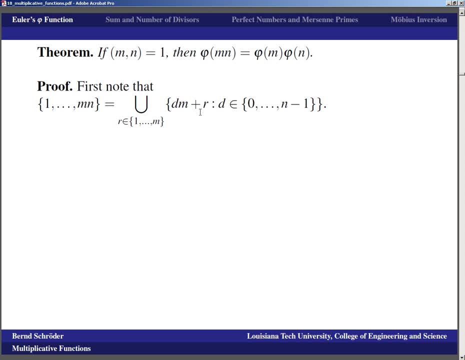 where d is between zero and in minus one. so this starts with d equals zero articles, once it starts at one in wendy's in minus in, in minus one and artists. and then we actually also capturing and we capture. all well, if the greatest common divisor of in and are: 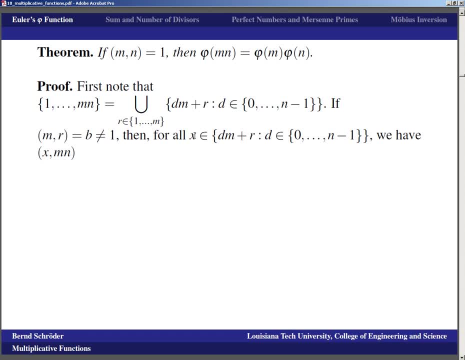 is being or equal one. well then, for all numbers, x in this set, where the remainder is, are. we have that the greatest common divisor of x and in times in is greater, equal than b and that's greater than one, and that is because any number in here 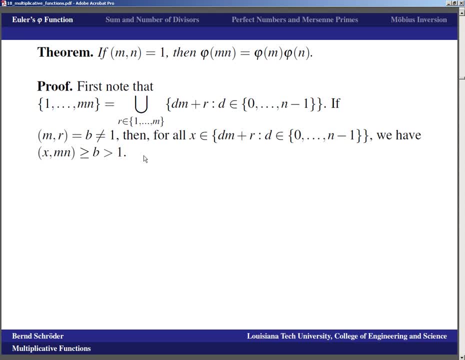 greatest common divisor between a number, dm plus are and and will be at least the greatest common divisor in are, i will be at least a race called advisor in and are, because anything that the by so stupid also to fight in and in in peter said already. so that means these are numbers. 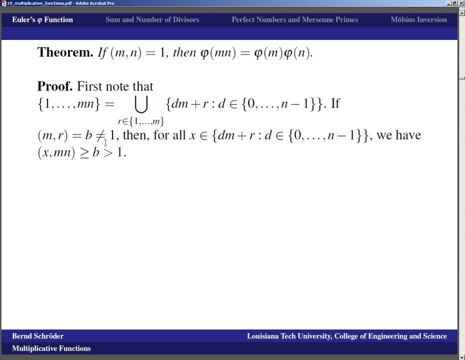 that are not counted by orders fee function, and so that means that certain remainders are simply excluded, namely all the remainders where the greatest common divisor between in and are he's greater than one. if the greatest common divisor uh of in and are is one, 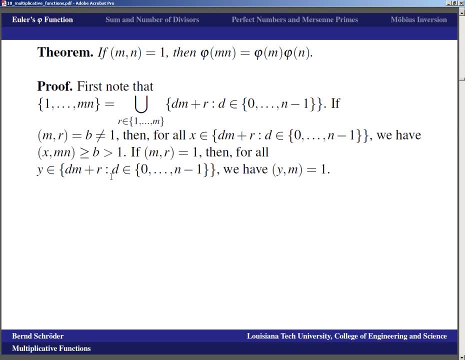 well, then again we look now and all the elements in the set in the city in class are ridiculous: from zero to you, in minus one and four, all these numbers, we have that the greatest common divisor of why indian is one and that is because otherwise, greatest common divisor of r and m. 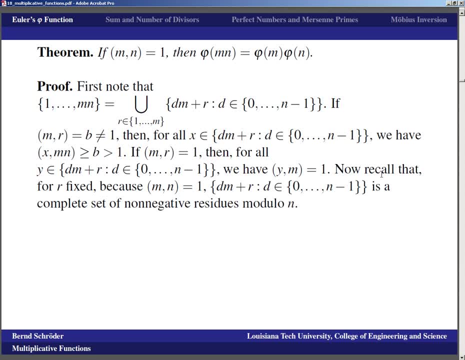 are greater than one, yeah, sure, and uh, now we would recall that for fixed are, because we assume that the greatest common divisor in and is one we have that this said here- is a complete set of non-negative residues. more to do it, because what do we have? the d? 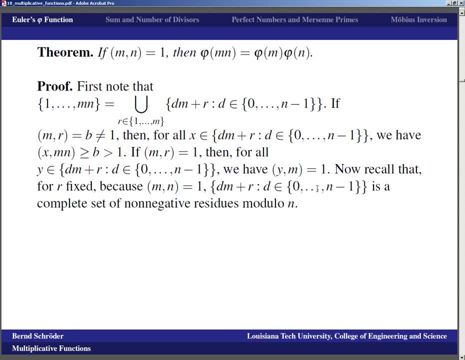 these are a complete set of non-negative residues module, in that we have to be results proved earlier, which says that if we multiply that with a number that is greatest common divisor, one within, if we had another number, we retain a complete set of non-negative residues. more to do it. 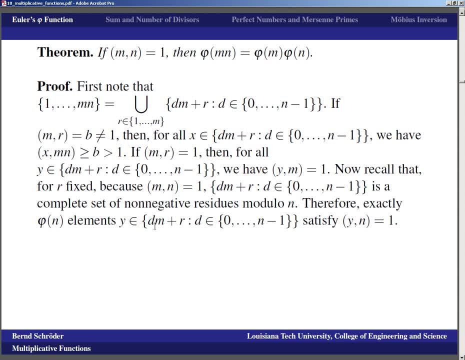 and so that means exactly field in elements of this set, dm, class, rd, from zero to in minus one, exactly few of them of these elements satisfy that the greatest common divisor of why indian is one because the greatest common divisor of light and its wanted it's called. 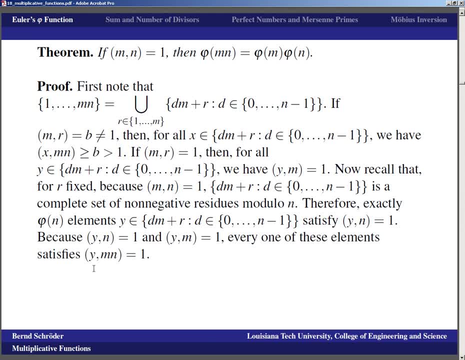 plans for a flight in this one, every one of these elements, and satisfies that the great mosque on the plaza of w�� in times in is one ins. that's all the rights that are ready, because there are few of him, since among these sets that we have up. 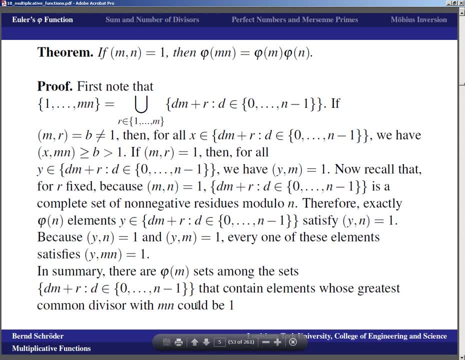 here that contain elements was greatest common divisor would in and could be one in each of those sex contains exactly few of in such elements. so that means to be, i mean is one point, is one a whole tax and one that the total number elements I in this set that have greatest common divisor one. 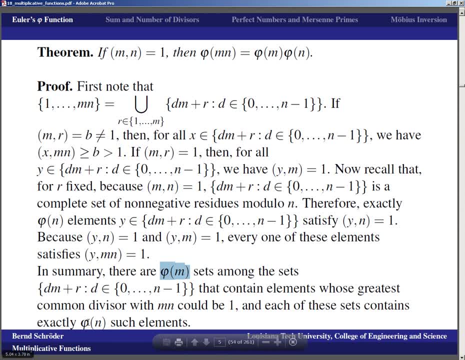 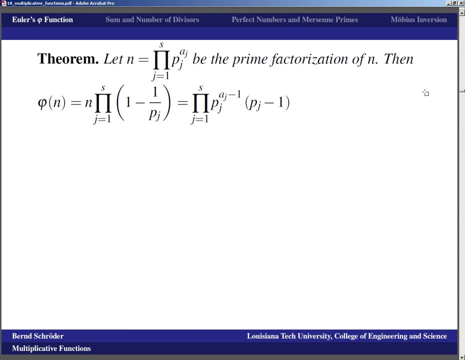 with in times in the East, feel and times feel, which is exactly what is claimed up here. and so, yeah, that's what we're saying and that instant, all right. so basically what that means is that if we have the prime factorization number in given, well, then we can write down: feel in its. 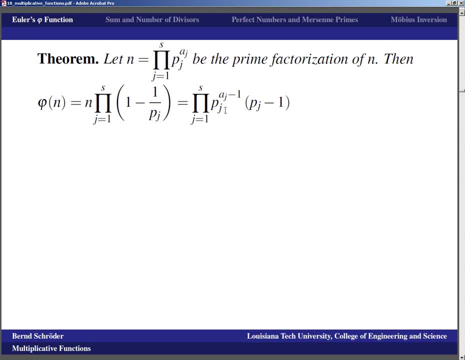 product directly and on it. see, the one that we're actually going to prove is this one and that basically says that, well, we can take the product out and we know that few pj2- the AJ is pj2- the agent minus pj2, the agent minus one. 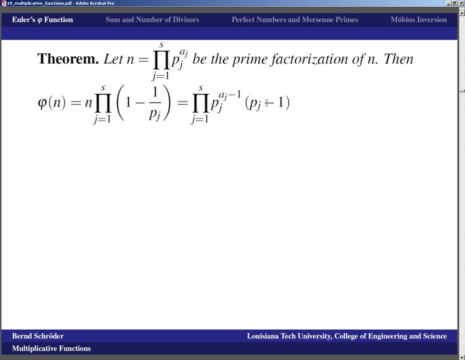 and if you factor pj2, the agent minus one out, you get this. so that works. and well, if I were to factor another pj or fear would get one over one minus one minus one of the pj, but then i could split up the product and the product of the pj to the aging. 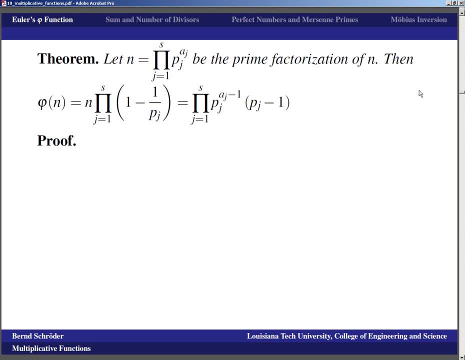 would be this in out front. so this is just arithmetic, okay, so how do we prove that will probably in action? in the base step is an earlier theorem that we have just uh shown, and so the elections that this test was one shouldn't be that bad, because 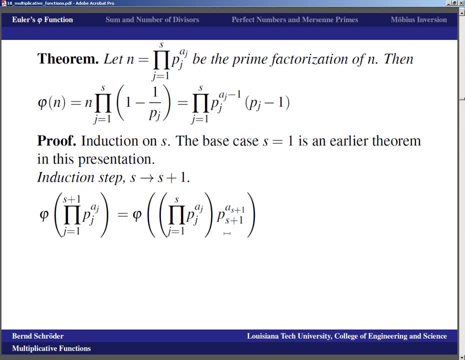 well, we take feel of the prime factorization. we split off the last factor, use multiplicity, because p s plus one has grace come to find one with them remaining product here. so this is feel of the product of the first, is prime powers times, feel of that. 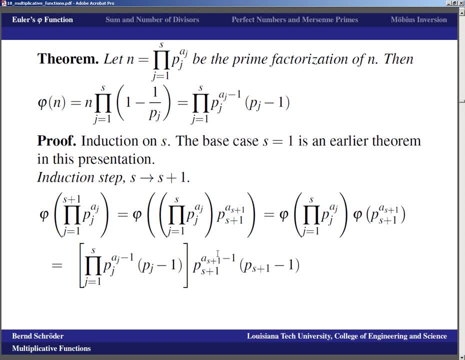 last prime power. then we use the induction hypothesis, which is that feel of this product is actually the product. pj to the agent minus one times pj minus one. also use that theorem and we uh split off p? s plus one to the a? s plus one minus one times p? s plus one. 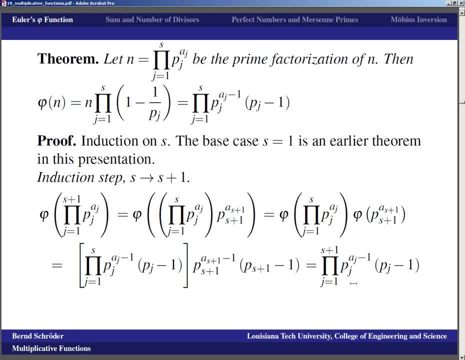 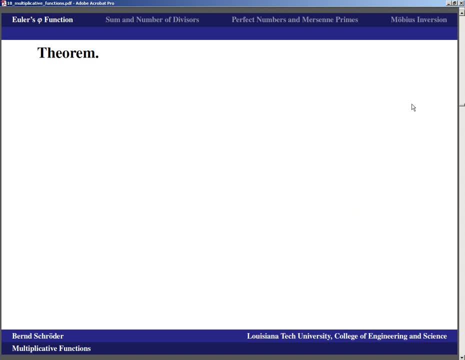 minus one, and now that is written x. after we combine the products, it is written exactly as it should be: the statement, and that's already so. uh, if we have an integer that is greater than two, then from this formula we can claim or prove that field in is an even number. 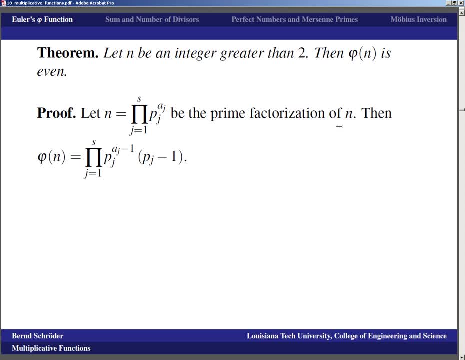 and uh, well, we look at the prime factorization of our number and their to. uh, well then, we know the few opinions. to practice equals وجets, pечb. eight minus one, pj, taxpages minus one. in there too close abilities, maybe you could have it ought prime factor: pj. and if that 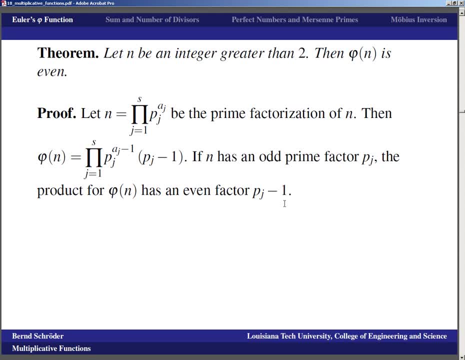 happens. well then, the products for fear of and has. see, you can talk to p j minus one is. so when is even? and the other possibility is that it has no walk insanters, and that means that in is true teh k in, because in was greater than two. that would mean that to to the k minus one is. 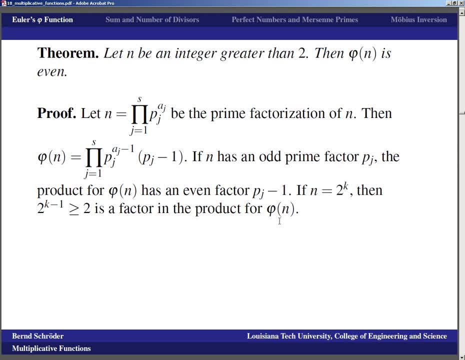 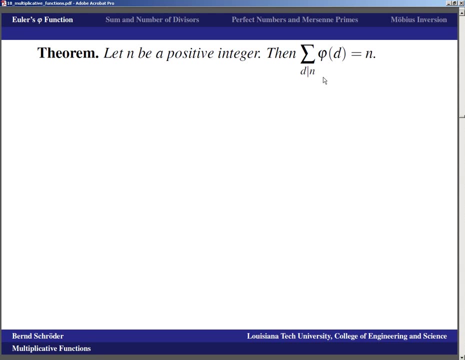 greater equal than two, and that's a factor, and this factor here in the product for fear. so, either way, as soon as in this greater than two- uh, few things and number, we can also talk about what we will ultimately call for summation function with a summative function. i'm not quite sure on the way right now. 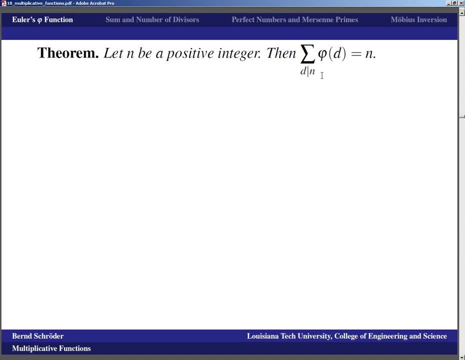 off the order fee, function it. what can be proven, but we will prove, is that if you've got a positive integer in into some over all the devices deal of in you some of the function fee of deep, you retain it and again that that sounds like it it. it ought to be ok, because some of those numbers ought to. 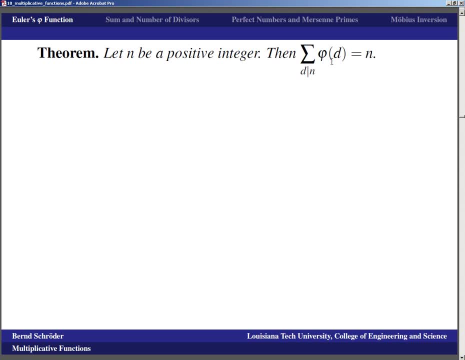 capture all the numbers below in? well, not not really, because the divisors are smaller than in, and so, uh, certain numbers, such as in minus one, would not not be in the sense that we're using to compute these fielding. so it's not entirely obvious, but will. 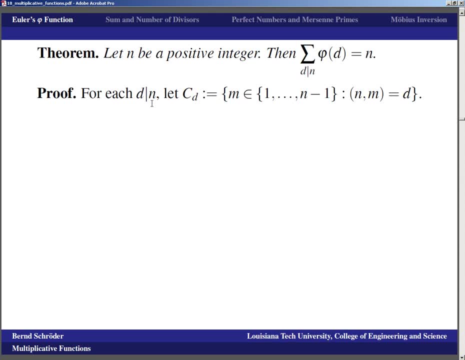 go through the proof. so, basically, for each divisor deal of in the world, it cd be the number off all numbers in between one and in, minus one, so that the greatest common divisor of in, in, in, in. what we know, then, is that the set of all numbers from one through in. 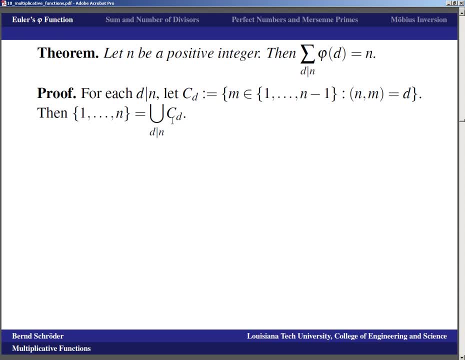 is the union of all the fighters. d off in c sub d, and that is all right, because if the if a set is is used twice, well, it no sense being used twice because we've got uh divisor here, uh, and we're looking at greatest common divisors, all right, so let's see, take 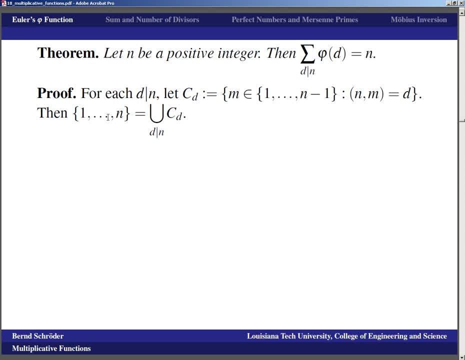 any number, uh small, smaller than that would be a number number in into that number in has a greatest common divisor, g, within, and so it's one of the cds right in. if you take a number in these sets, uh seesaw d, well then of course it's a number between one and minus one. so that's it. 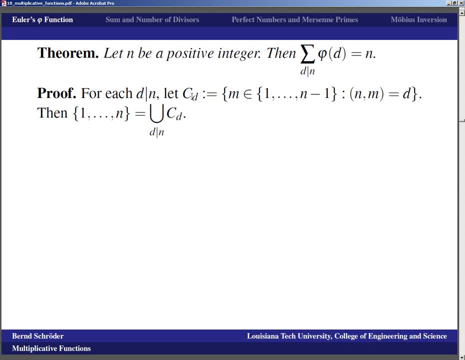 here and i would say that probably see something in that's going to be just singleton in. so we probably have to assume you see something that's a single and so well, or this is just a set one, two in minus one. i think that should be said. 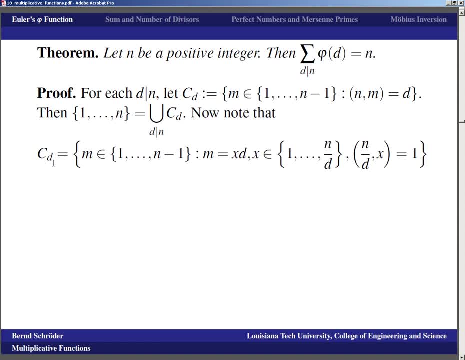 once we okay. so now let's note that c sub d is a set of all numbers between one and in minus one, and so that in the six times d, where x is a number between one and in over d and the greatest common divisor in over d index is: 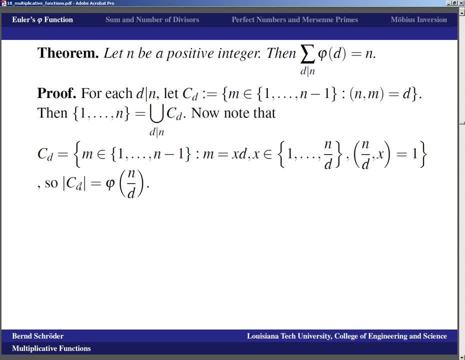 and that means that the number of elements off c, sub d is actually often over d, and so that means that in the insta some off all the d dividing in ceaser uh, cd absolute value, which is to some overall d divided simply off and over d. 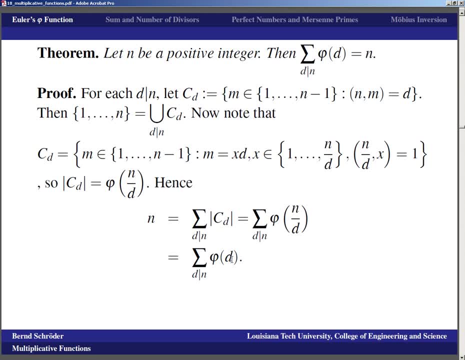 and that's the same as some of the divides in fee over d itself, because we some over t, in over the. so whether we saw the these when that the device, our and and in over t ucc, defizer, and i think what we treaty say here. 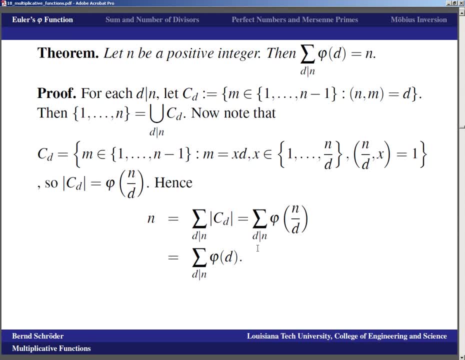 is: uh, that fee off used to be separate and and i think we simply have to go up to in here. hang on just a second. uh, yes, indeed, yeah was a little typo on these slides. this, it's c sub d, consist of all the numbers in between one and in with. 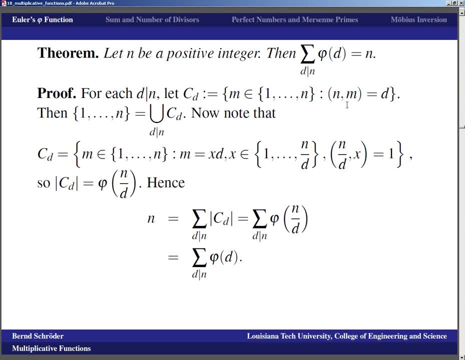 graceful divided d uh with, with in and uh. that certainly means that the sets of seats of the or pairwise disjoint, because the greatest common divisor is unique. uh. it also means that the, the set from one through in, it's the union over all the cds, because every element in here 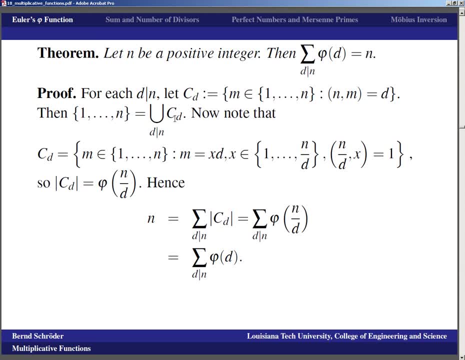 use uh in one of the cds in the d that uh is the greatest common divisor between it and uh in and uh. that's then me and now the rest is okay. here we're looking at at the six cd old former pettis at all numbers bigger where need in? 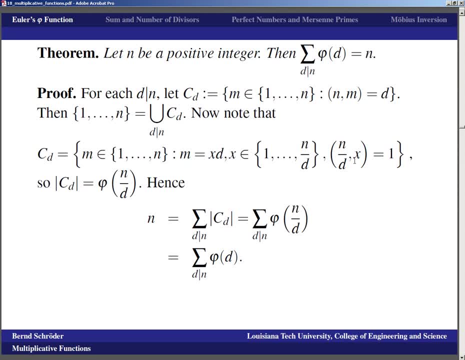 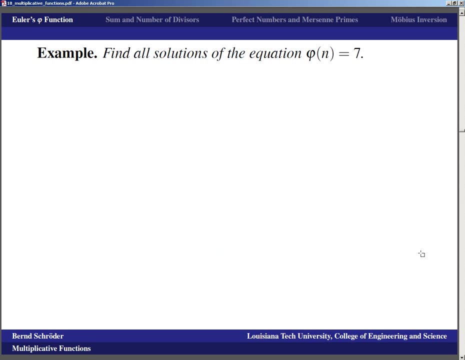 so that in his details, x-ware, the greatest common divisible, exit in to find all solutions of the equation field and equal seven. well then, because seven is not, even if you have to, is one, there is no solution of that in. uh, for even right-hand sides, that argument. 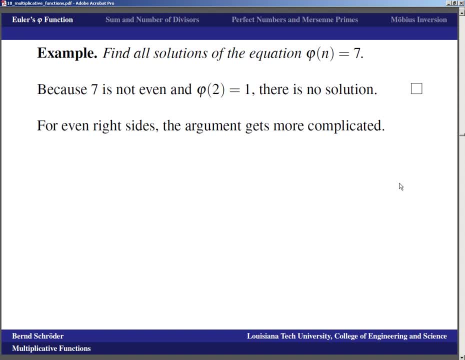 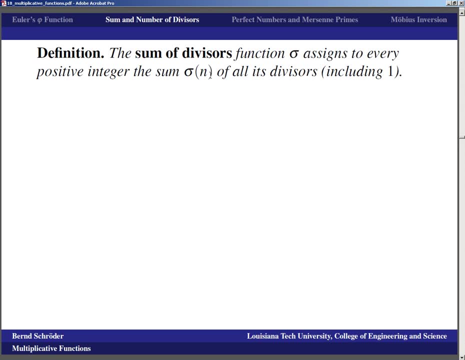 does get more complicated, and that is something that i'll leave to you. okay, so now we're going to talk about the summit number of divisor functions, the- some of the fighters- function sigma assigned to every positive integer, to some signal in of all its divisors, including one. 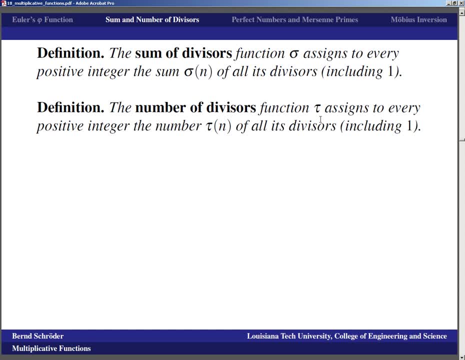 int uh. the number of divisors function tell assigns to every positive integer the number- how often- of all its divisors, including one, and i will. we talk about the visors here. we certainly only mean positive divisor, so it would be the numbers between one and in. 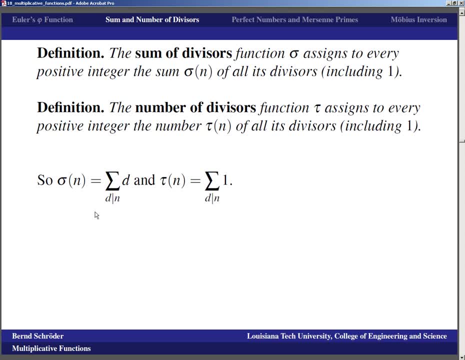 that can be used as divisors. so basically what that means is that signal of in, is that some fight of d and tae, cycling and becoming, or is the sum over all device in off, one built very similarly to what we have seen in this format for the order of evоп. 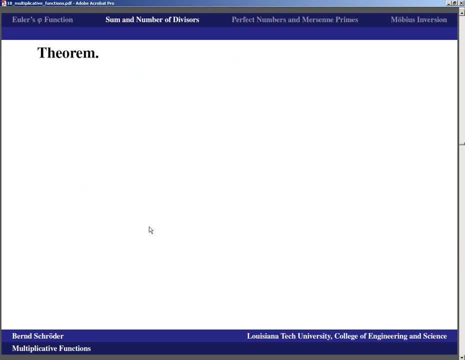 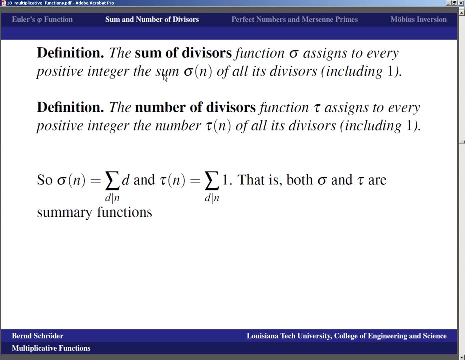 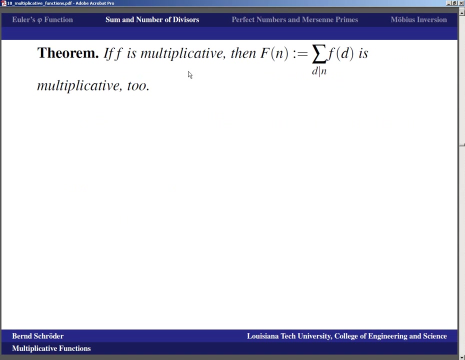 and off. that means thatiset both sigma channel are what it's called summary functions. witch we october twenty-eight. okay, the summary function is what you get when you take a function function at. in this is some overall divisors of him, some other, and so now we're going to talk about these. 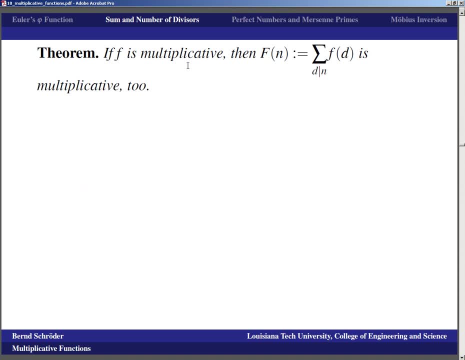 summary type functions a bit more. and if a function, if it's not to pick it up, well then we define it for him to be the some over all these at the fight divides in if of the where we have a cabinet for the summary function in reclaims that, if ever small, to pick it up soon. 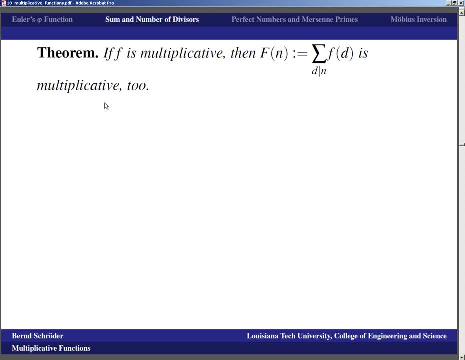 capital f. the summary function is not to kick it too, and uh, in fact this is actually in if and only if, but we're going to need movies in version or to prove the converse. so right now we're just going to assume that lower case x multiplicative. 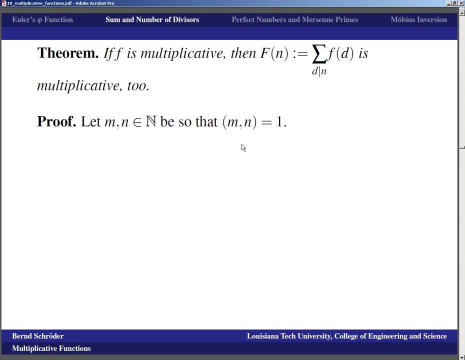 info: multiplicative eddy, we remember we need to take two numbers, eminem, so that the greatest common divisor of these two numbers is one and uh. we want to find if, often times, and of course capitol m times, and well, every day, every national number x. 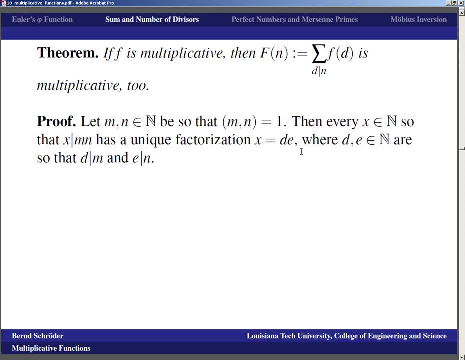 so that extra bites in times and has a unique factorization d times e with the in your natural numbers, so that the device in the device in, and that is because in and in don't share any, and so that means, if i take it within times effort. 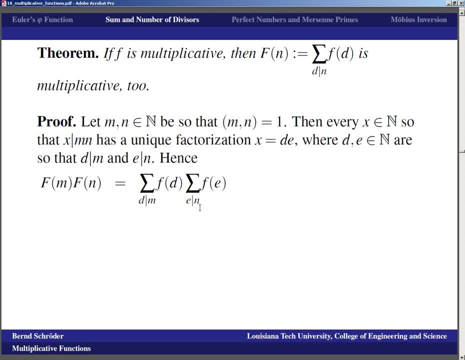 well, that's the sum over all these at the buy-in info d plus a sum of all the that divide in info. you and i can pull the sums out of it if of the times before he. now these two don't have common divisors, so that means if of the concept of the. 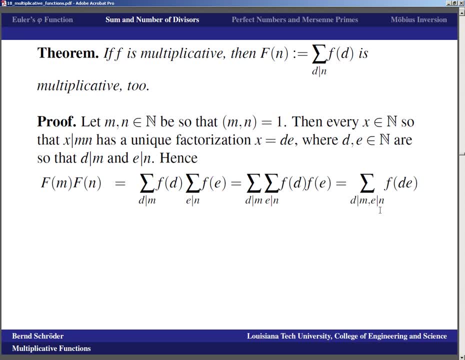 use of the times. he had to some mistress over all. do you think if i didn't get by it dividing in, if i already have a multiply together, then when i saw more of these at the vitamin or you could divide in? i'm basically just something overall divisors of in times, and so this is some. 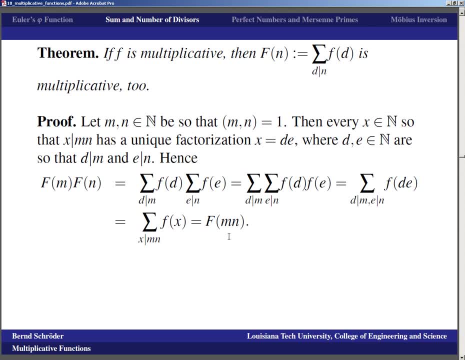 of our all, x dividing in times, in if, effects, and that's capital f of in times, and and, and that's already it for this i have a theory of here, and that he has that sigma, and tell our multiplicative, and yeah, that's because they are both these summative functions, right. 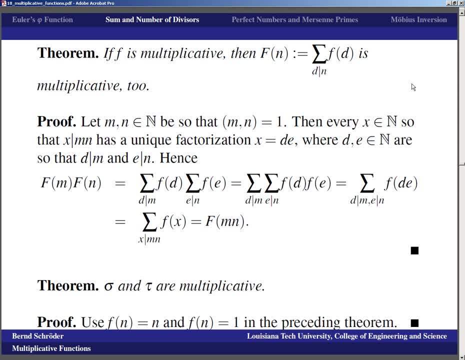 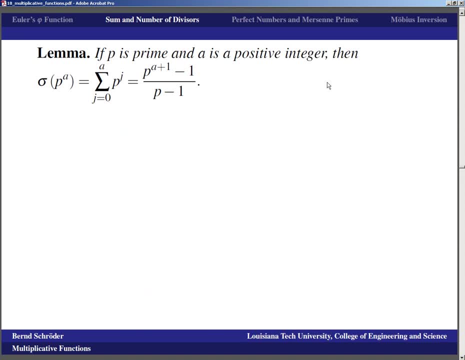 united xo pen. equals an equal thing was one of the preceding. okay, so now we have an emma and we also, just like we did for the order of the function we want to see if we can't compute. these functions are fine formulas and so it is a prime number. 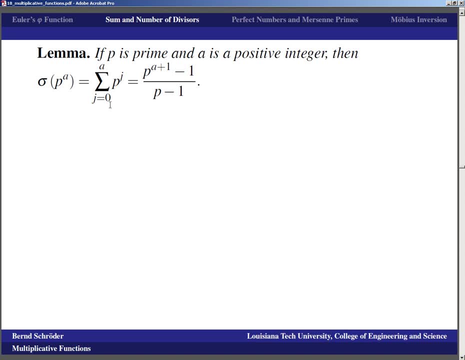 and a is a positive integer. well then, sigma of p to the a is the sum j equals 0 to a. p to the j, it's the sum of all divisors, and that by the sum for geometric sequences is p to the a plus 1 minus 1, over p minus 1. 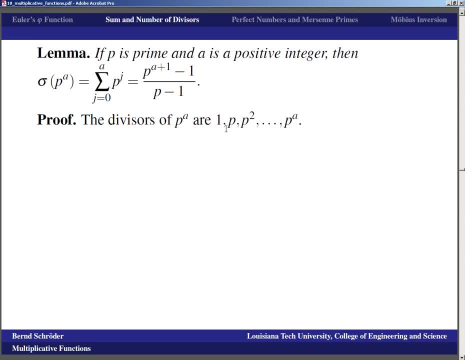 the proof is basically right there. right, the divisors of p to the a are 1, p, p squared, and so on all the way to p to the a. and that means the sigma of p to the a is the sum from j equals 0 to a, p to the j, and that's p to the a plus 1 minus 1 over p minus 1. 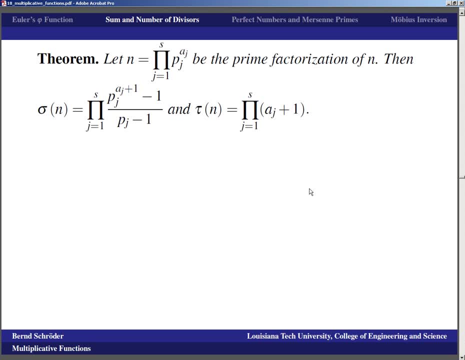 that means that we can actually write down what these functions are with a product formula, namely if we take the prime factorization of our number in to be the product p j to the a j, well then sigma of n will be product j equals 1 to s, p j to the a j plus 1 minus 1 over p j minus 1. 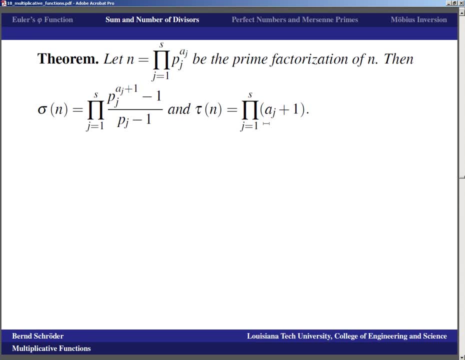 and tau of n will be the product. j equals 1 to s a, j plus 1, because well, we're going to have a setting y, j plus j. Bureau of progression. we'll see you in a minute. pj to the a, j has agent plus one. 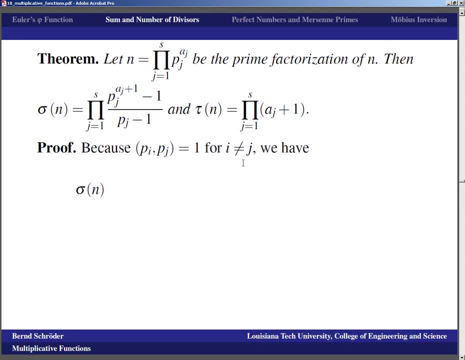 quite simple. p, i, p, g have greatest comment about the one, for i'd like to jay. so that means that signal of them signal off. j equals one, two years pj to the a? j, which for a lot of negative functions is the product. j equals one, two s sigma pj to the a? j, and that's the product. 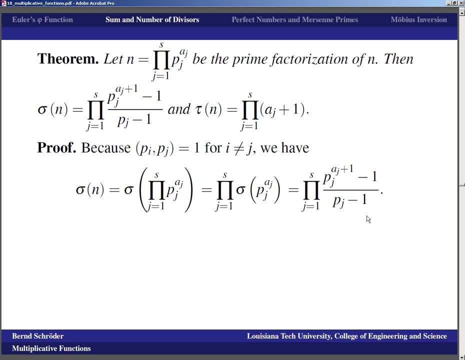 j equals one. two s pj to the a j plus one minus one over pj minus one. info: tell. we use the same argument, only that tell pj to the a j is a plus one and that means this. proof is that now we're going to talk about. 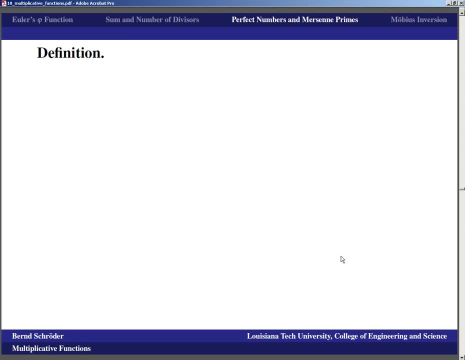 perfect numbers and person prime numbers, and so this is something that again goes way back to the ancient greeks. but then mersenne prime numbers are something that people are interested in because it it pushes again, uh, boundaries for primality testing. so a number is perfect. 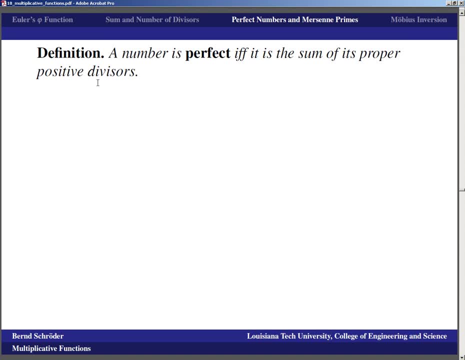 if, and only if, it is the sum off its proper positive divisors. and that is the case if, and only if signal of energy put it to win, because in itself he's also one of the device, right. and so now there's a theory, and the theorem says that in even positive 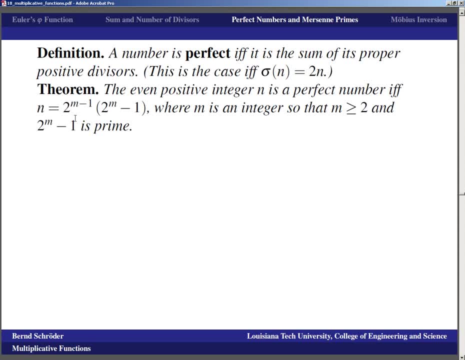 integer in is a perfect number if, and only if, it is true to the in minus one times two, to the m minus one. verbally that doesn't sound like a different, but in the first one the m minus one is in the exponent right. where in this integer? 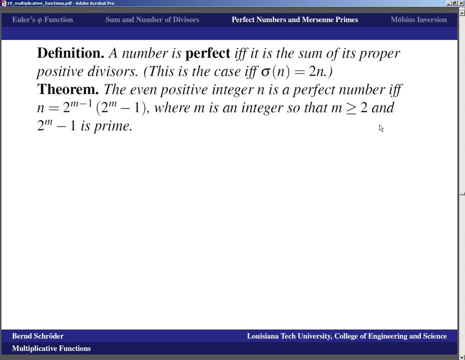 that is criteria k gelen to be, because we have to make sure, see, but right, and we have to make something. show that to to the in minus one properly. i'm going to say that they are on also, but my school c плюс u views that these: 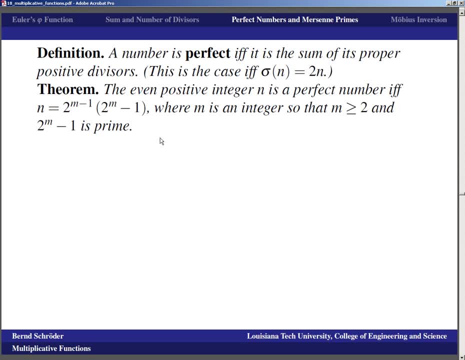 they're also is a characterization for all right perfect number spot dot. please, beyond our retrain elk a. so what's the proof? look at numbers off the form two, two vm minus one times g. we're just going to go to the, which is all it can in this greater equal than. 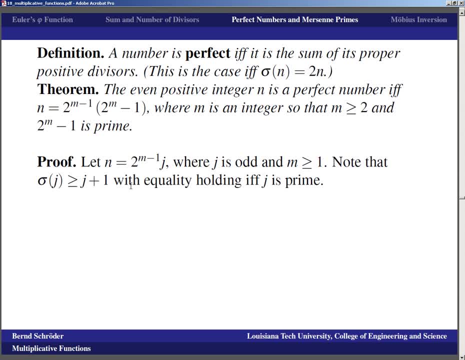 well, signal of jane is greater, equal than jay plus one, equality being true if, and only if, j is prime right, because, uh, if j is not trying to be get more here in it, if we get this exactly, then jay must have been prime uh in. if they take time to get exactly this. 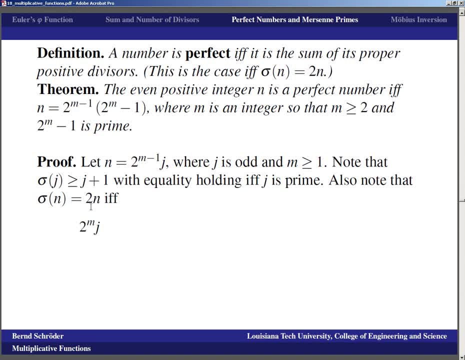 also, we want to note that signal in is equal to in if and only if. well, okay, we already knew that signal, then it's good to wait for me. if it's prime, so this is just perfect, and so this is just another way of saying that in is. 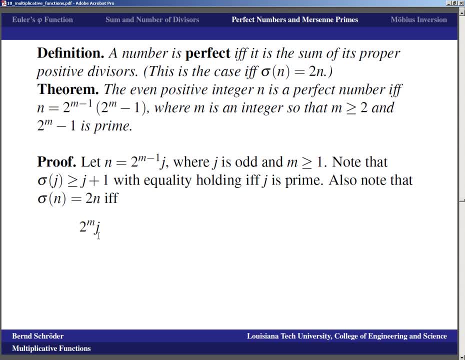 perfect, and that's the case if, and only if, we want to look at to to the end times j, which is a good looking, that's two times to be a minus one uh j, which is signal off to to the in minus one times j, yeah. 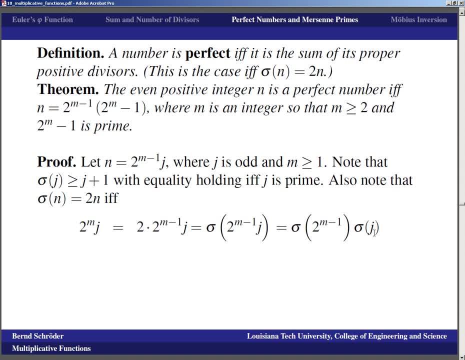 uh, and we can break that up. that is signal to to be a minus one times signal j, and signal to to be a minus one is just to to be a minus one. we've just shown that our proceedings like. so that's to be a minus one. 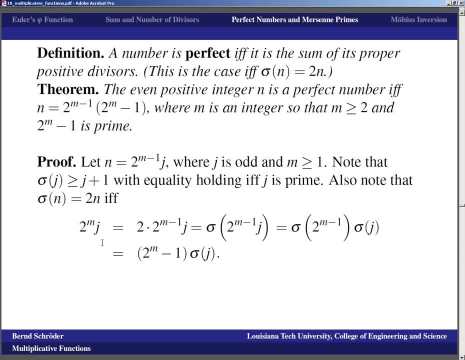 signal of jay. so that means in this perfect if, and only if, we have this equation here and now for the direction right to left. so, assuming that in is to to be a minus one times jb into to be in minus one, we go right to that. 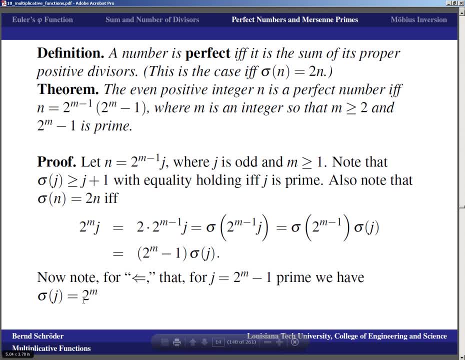 left, and so for j equals two to the m minus one prime. we have that signal of j is equal to to to the m right, because it's number plus one, and that means that the equation holds because now we have that j is to to be a minus one. 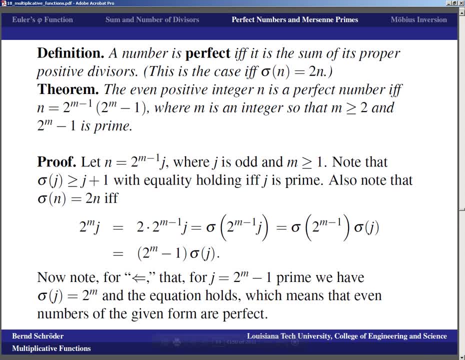 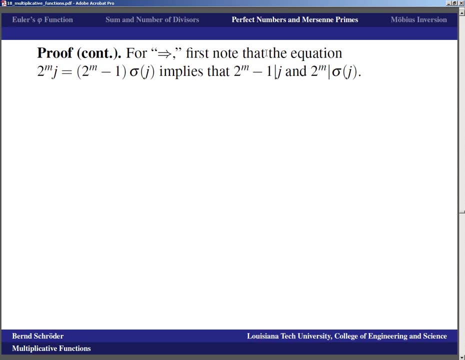 and we have signal jb into to the event already means even numbers off the given form really are okay. now we have to prove the other direction. for that we go to the next panel, and so for left to right we have to uh, take the equation that we have, that said, that the number is perfect. 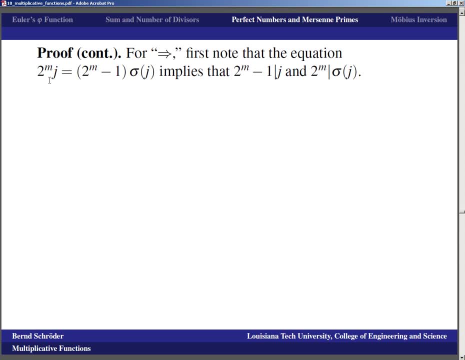 uh, if, and only if, this happens. well, we now need to find consequences of this equation. and so, if we're looking at two to the m times, j, equals two to the m minus one, equal signal j. that applies to two to the m minus one defied jay, because no or number divides the power of two. 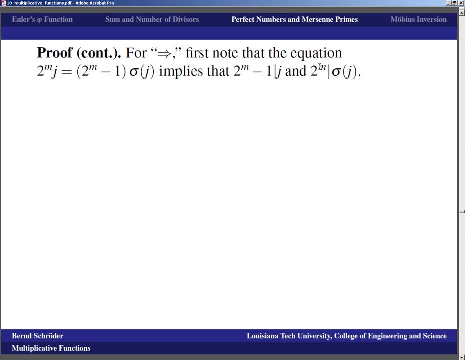 two to the m device signal jay, because no power of two device, any i'da vice an odd number to to the m one's what. okay, so that means that j eight years to two to the m minus one times some deep, and signal j this to to the m times some heat, if we can just proof. 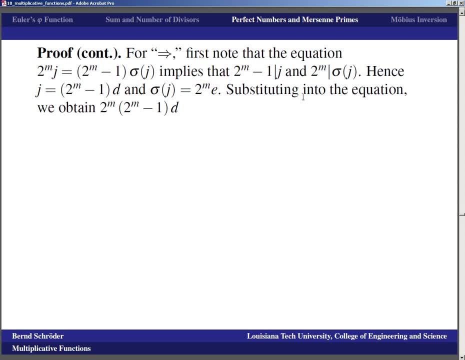 that the Wilson equals one, we ought to be ok. and so if we substitute into the equation of u b, two to the m times two to the m minus one is zero over j. two to the m minus one, d as to the end, and that on the right, now that you can, j. 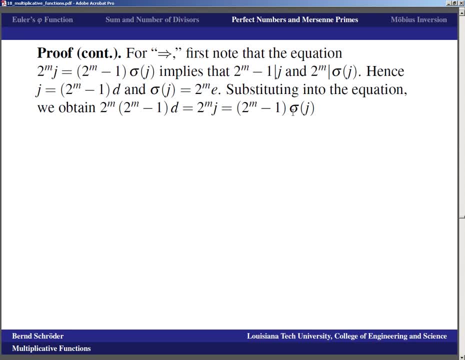 which is to to be a minus one signal of jay- and signal of jay was to to be in the east of this- ends up being to to the m minus one to to the end times. he and we can see the cancel and that means that we already have. 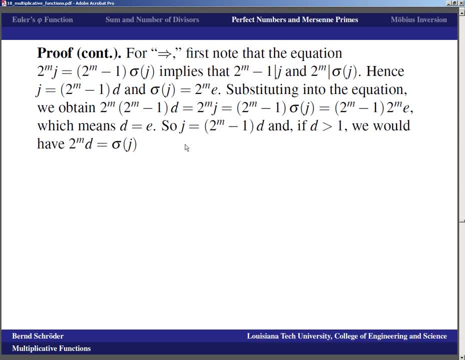 that d must be equal. so that means that j is equal to two, to the m minus one. d again is where now need to check what happens if he was greater than one. and we're going to find the contradiction there, because what do we get if d is greater than one? 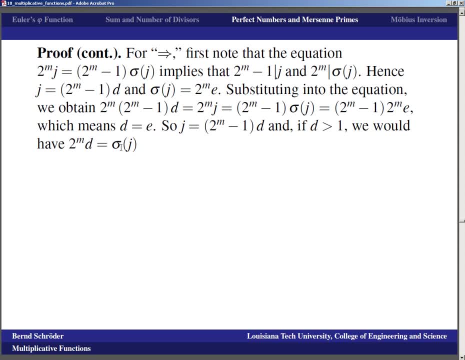 we would have that to to the end times. d is equal to sigma of j and uh. that would be: uh, yeah, that's because j is to to the end minus one times. these will be pleaded in here and cancel the two to the m as well. so that would be. 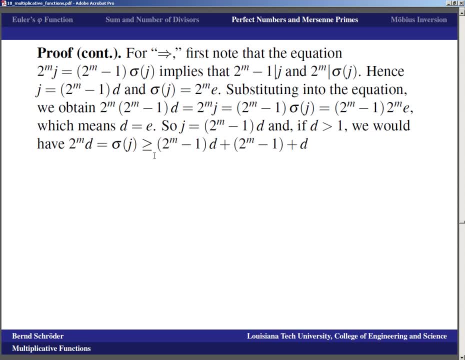 to to the end times. d is sigma of jay, signal of jay, yes, signal j is great. repose in to to the end minus one times d, which is a number itself plus the other two divisors that we know. two to the m minus one. 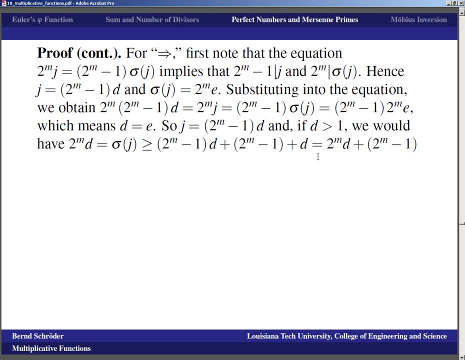 and uh, if we see that we get a minus t plus t, so that goes away. so that's two to the end times d class to to the end, minus one. and we can see that that can work because we've just shown the two to the. 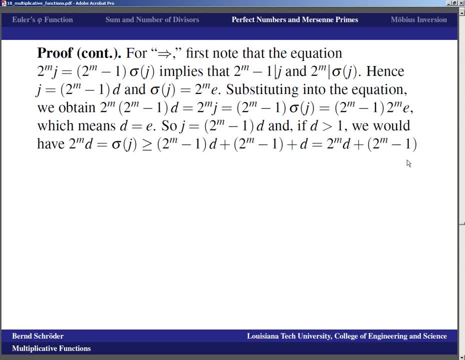 end times d is greater, equal than two to the m times the plus a non-native number, and so that's not possible. so that means that the use one and that means that j is to be a minus one in signal, j is to be in which is j plus one? 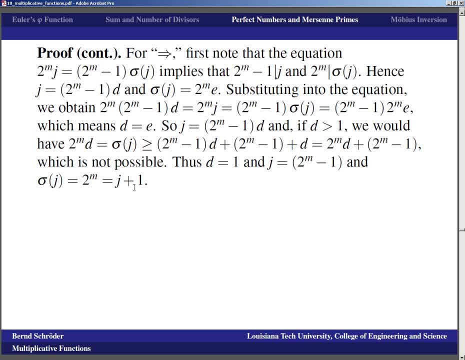 yeah, okay, so that's j plus one from here. okay, we now have, uh, the numbers that that in this off the right form, in this off the form, two to the m times two to the m minus one, and i felt like we're done. but remember the other thing that was said was that j was supposed to be prime. 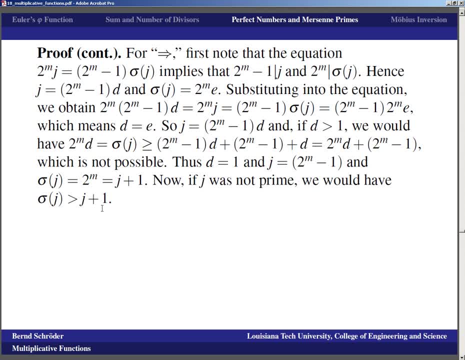 so if jay was not prime, well then we would have that signal. j is greater than plus one. but we had already seen here that signal of jay was two to the m, and so that means that j equals two to the m, minus one is prime, and in videos all the way, 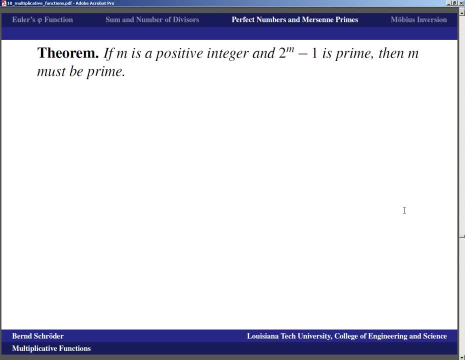 as indicated. and well, if in the is any positive integer and two to the m minus one is primed in, in must be prime. so because people were interested in these perfect numbers, people became interested in these factors that we must have. so a natural question to ask you, given with, given from the 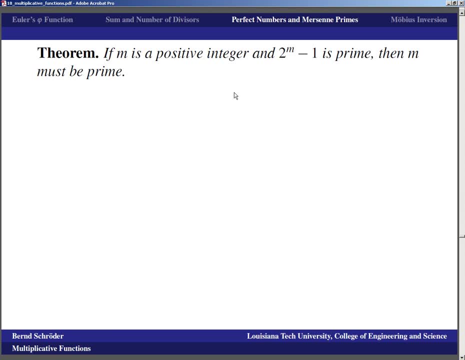 previous theorem is that if two to the m is prime, what must in the end? well, we kennedy's concluded in must be prime, and that is, if in was actually a composite number with non-triggered prime, non-triggered factors p and q, then we would have that two to the m minus one is two to the p to the q. 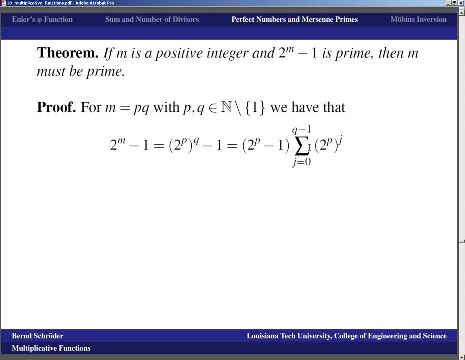 minus one, and that is two to the p minus one times some j equals zero to q, minus one to the p to the j, and that is usual formula that you have when you take a power minus one, then that is the base minus one times. uh, this kind of summation. 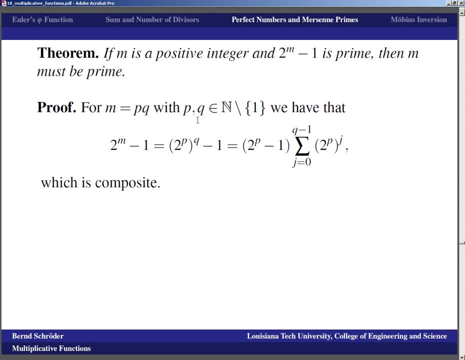 and that would mean, of course, that that is composite, because p was greater than one, and that handles this one. so definition: the number in southern, which is just two to the m minus one. so it's really not terribly strange looking thing, but that thing is called the mth merson number. 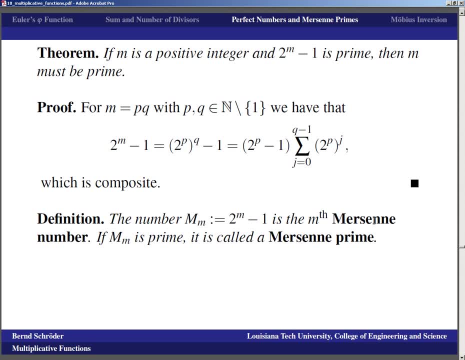 uh, in honor of the french mathematician named merson, who probably not necessarily prove that one, but probably prove the serum before that. not quite sure, can't. can't say that i'm not a historian either. uh, and, if this number in something is prime, we will call it a. 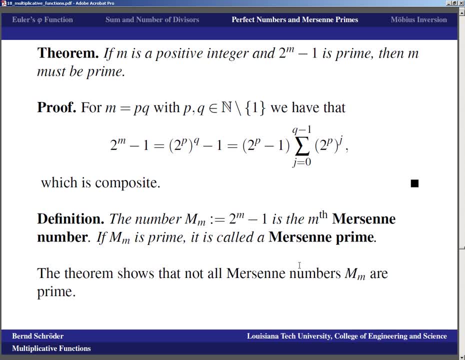 mersenne prime. the theorem up talk here shows that not all mersenne numbers are crying. but even within this prime in something need not be trying. for example, if we're looking at the number in sub eleven, that's two to the m minus one, and i know what that is. 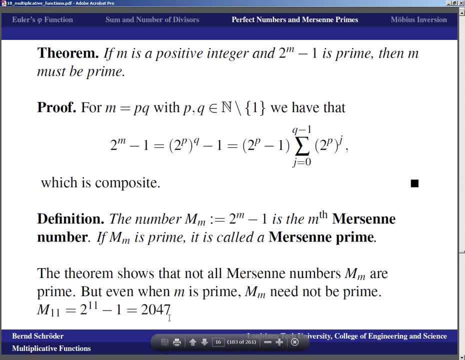 two thousand forty eight minus one, so that's two thousand forty seven. the part that i wouldn't necessarily know directly is that two thousand forty seven is twenty three times eighty nine, and let's see how would that go. uh, two times eighty nine is a hundred sixty years, a hundred seventy eight. so 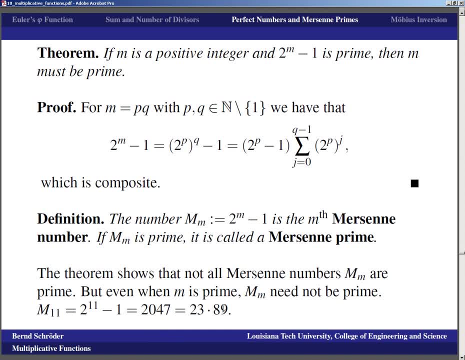 that would be twenty times eighty. nine, is seventeen hundred. eighty plus three times eighty, which is two hundred forty, would give us two thousand and twenty plus three times minus twenty seven, giving us two thousand and forty seven. so these things keen still be verified into more you train yourself to do. 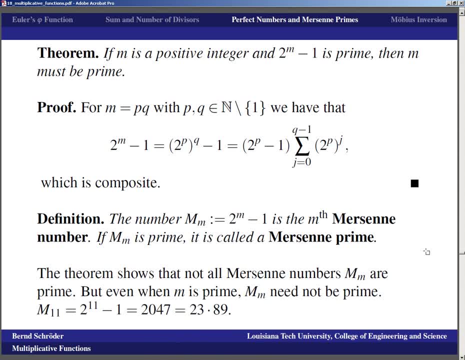 reasonable arithmetic also in your head. the easel easier these kinds of things will be is actually also the sharper your brain is overall, because actually, uh, we're now in the uh seventeen, three teens presentation, i think of record seventeen right now, cause i've skipped one. 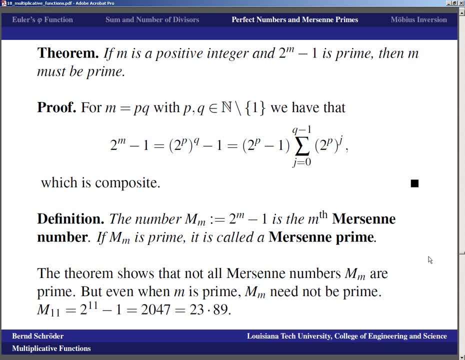 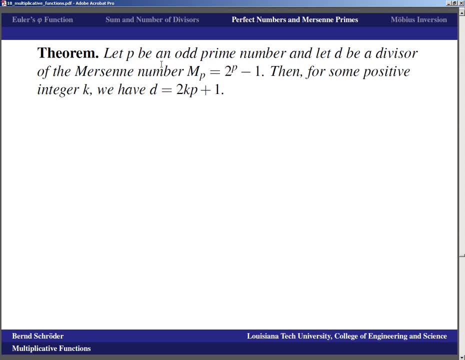 uh, and i'm there while charbert with numbers that i was at a start at these things out. well k, let's talk about trying numbers. uh, so if p is not prime number and d is a divisor of the mercer number inside, p equals to two p minus one. 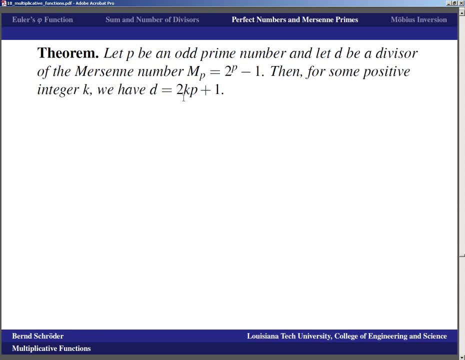 we claim that for some positive integer k we have that d is to k p class one. so basically the divisors off mercer numbers that come from prime numbers, that the one mercer number that comes from even prime numbers- not that interesting, it's three, all of the divisors. 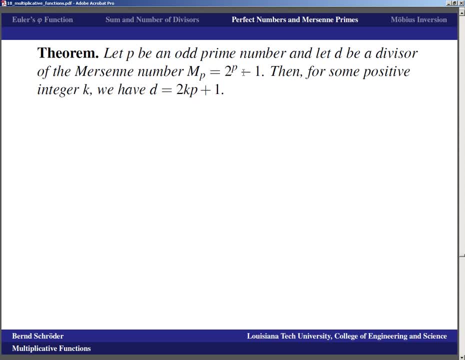 off mercer number set happened to mercer numbers that are national candidates to be primes but aren't must be of a very special form, namely they must be one off from a multiple of that exponent. okay, so that the devices. okay, so that you'll be a prime factor off this number in some people's 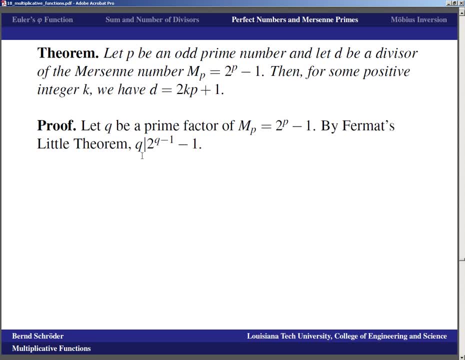 two to the p minus one. well, by fair must little theorem q itself divides two to the q minus one minus one. yeah, that's because two to the q minus one is equivalent to one working new q, and so that means, at the greatest common divisor of two to the p minus one, in two to the q minus one. 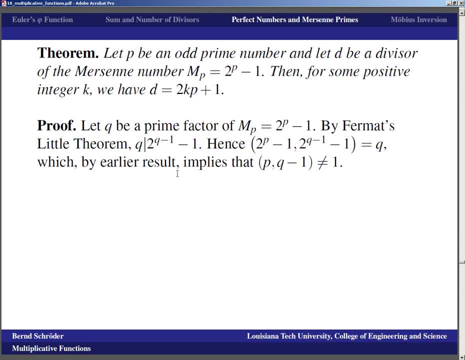 minus one is equal to q. ends by an earlier result which we had, which talked about numbers that were off this form, power, okay, our of two minus one, the greatest common divisor, if the greatest common divisor to of these powers greater than one than the greatest common divisor of the exponents, must. 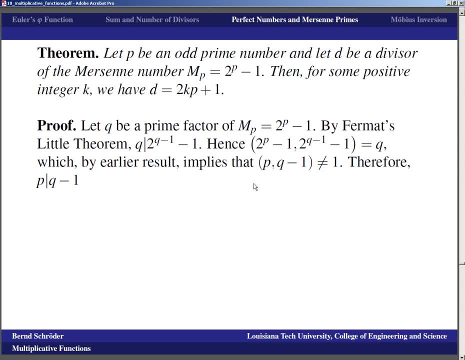 also be greater than one. and, uh, because he is a prime number, that means that he divides q minus one and that means q minus one is in times p and because q all i did, and that's because this thing doesn't have any factors. uh, we have that in this. 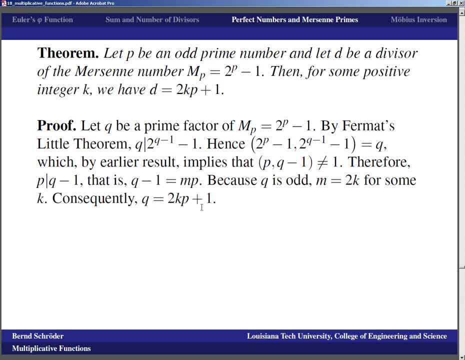 two times k for some k, and that means he was to kiki plus one. and any divisor of in sub p is of course a product of prime divisors, and that means it's been a really truly simple deduction on the number of prime factors with multiplicity. 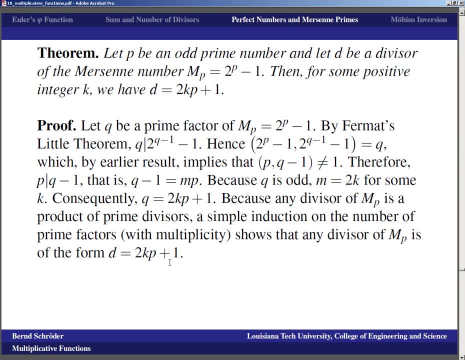 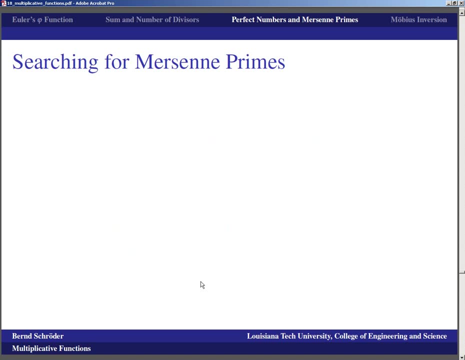 shows that any divisor of the mp is off the forty equals to k, p plus one, because anytime i take two numbers of this form and multiply them together, i get multiples of p plus a one at the end. okay, so that was a quick overview of of of perfect numbers and where they're sent prime numbers come from. 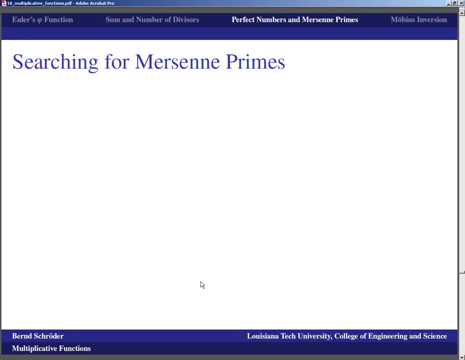 and uh, if you look at perfect numbers and don't consider them perfect, well, that is something that is, i would say, on one hand, traditionally, and again p for people who go nationally into number theory may really look that way. for an outsider, the beauty is in the eye of the beholder, certainly. 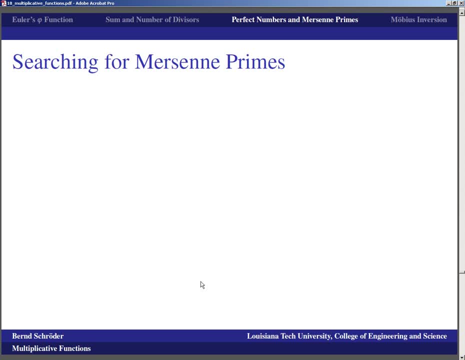 but uh, it shows that merce and prime numbers have any place in number theory, and so there's a search for merce and prime numbers and there is in fact and all of pq test for whether, for prime number p, the merce and number in sub p is prime. 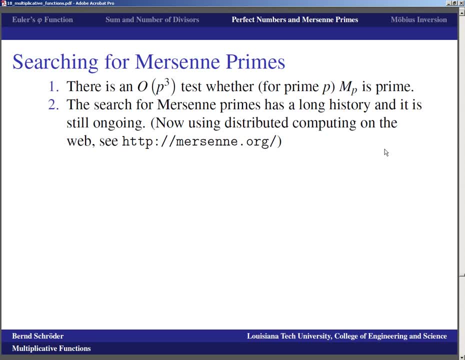 uh. the search for merce and prime numbers has a really long history and it's still ongoing. it's now using uh distributed computing and if you're interested in that, go to merce and dot org ends. it's really interesting. again, that's here we run into these easy. 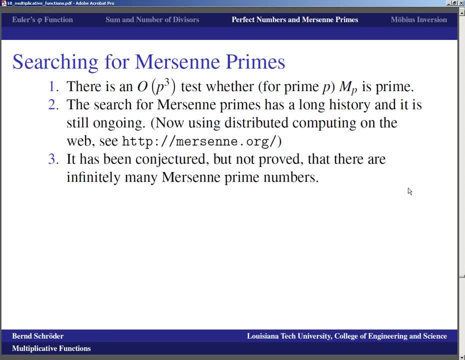 conjectures that ever in fact easy to you explain to people. it may not be uh as easy to explain to people why people are interested in mercy and prime numbers, but you could tell somebody with basic knowledge of powers, whatever sin pride is. it explained. the conjecture is that there're infinitely many merce and prime. 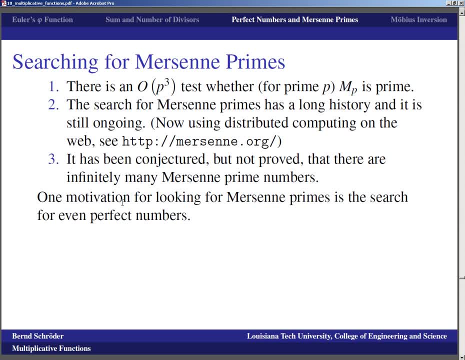 numbers, but it's not been proved. uh, and one motivation, one practical motivations, and out where one historical motivation for looking for merce and crimes is to search for even perfect numbers, or perfect numbers need to satisfy so many conditions. there are lots of things talk to them about why you have the family and society. there are lots of things to discuss, but they don't necessarily give you the answer for that. 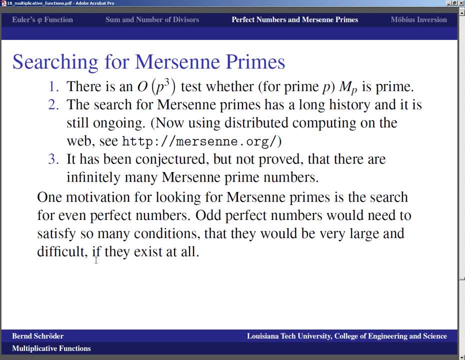 on the other hand, their whims that they would be very large and difficult, if they exist at all. so pay. it wasn't quite truthful with you at the beginning. that's again. i only play a number, theorist on this show: ice. i don't know where are perfect numbers are. 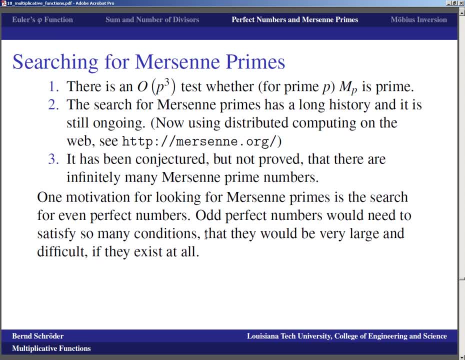 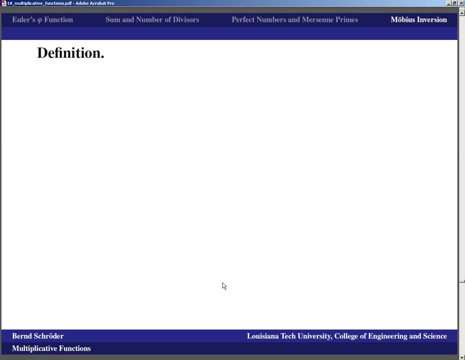 completely characterized, or if this just means that they found conditions and conditions and conditions, and that means that they have to be very large, if they exist at all, and the proof that exist, that decides their existence or non-existence, has not been founded. okay, so now we go to. 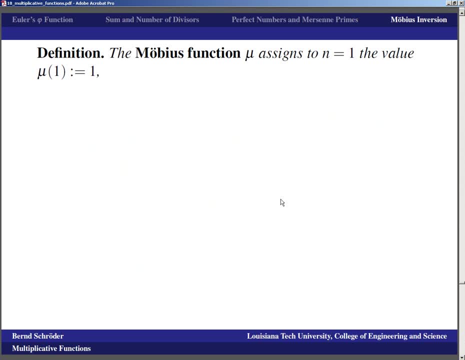 news in version. and that starts with the media's function. all named after the german mathematician. maybe isn't a pretty sure that's also the one with the media strip and uh that that maybe it's not going to be strange, right, it's uh called you. 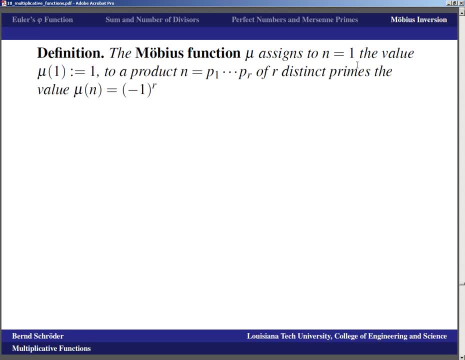 and it's assigned to the number in equals one, that that you, you equals one equals one. and for any product of artistic prime number, it's it's science if and you have been equals negative, one to be or into all other. in it assigns the value you u of in equal zero. 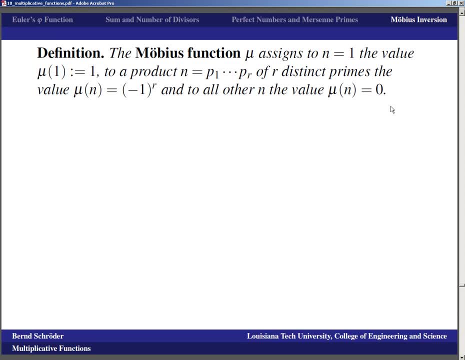 and i have. this is another one grand, typically saying class at no matter mediation store. just follow the billions a business when i'm going to find in as far as i could see from as i prepare peace lights, the motivation for why he would have been interested in dysfunction comes. 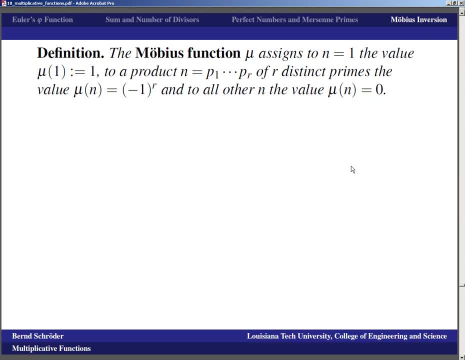 probably from the last proof on the slides will be proved that if the summative function is multiplicative than the original function is multiplicative also. so first we just prove a couple of results about the movie is function, and one of them is that the movie is function is. 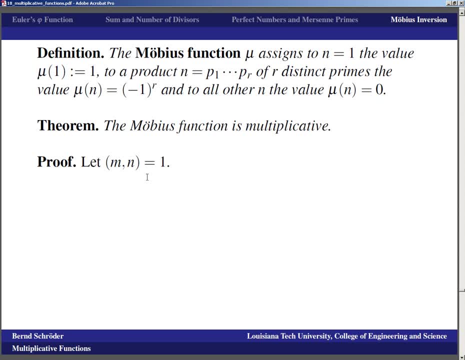 multiplicative itself. take two numbers whose greatest common divisor is one. well then, multiplicative use, multiplicative t is trivial if one of and more in is one right, because then the product is just the other number. in new york one is one also, so nothing happens. if you look at this zero, new york is zero. there is a repeated prime factor in. 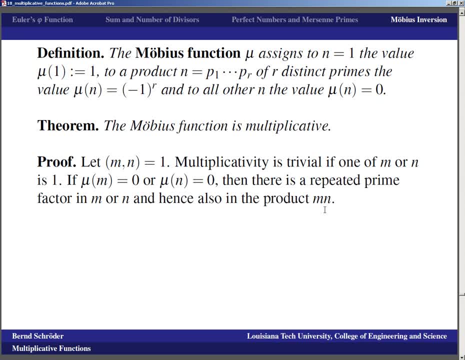 a morning, and that means there's also one of those in in times, and so that means both sides are zero. so in this case, with new york in this equal zero which is new york and times new york in, indeed, if new york and is not zero at new york, in is not zero. 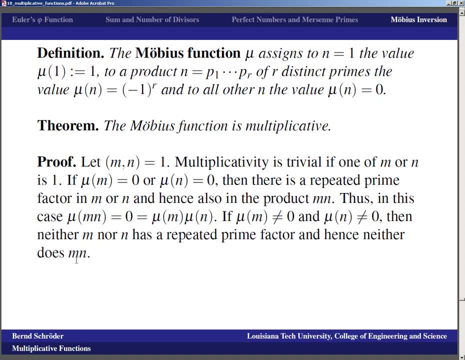 well then, neither of the two numbers as a repeated prime factor. it hence neither does in times in, because, remember, we have that in times in, greatest common divisor is one and uh, then we just take are in to be the number of prime factors of a man are. 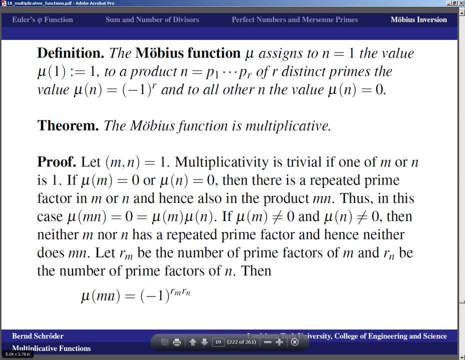 in to be a number of prime factors of in, and we know that you off times in is negative one to the are in class, are in, not times are in and we're back in your surplus. and that's, of course, simple algebra that's made of one. 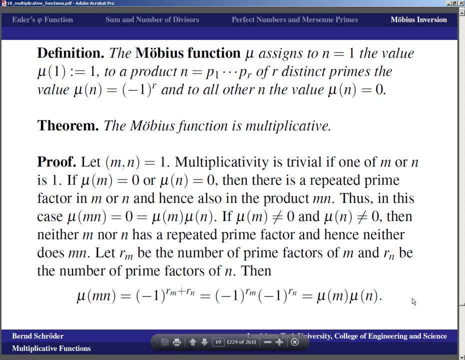 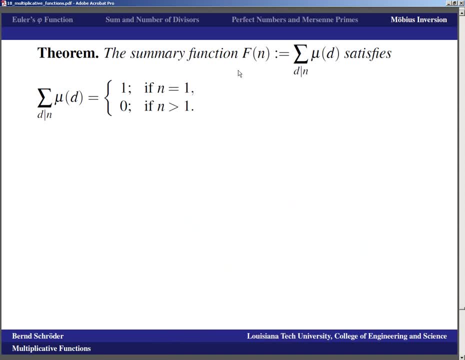 to the are in times, native, one to the are in, and that is new york and times and uh, that means that the movies functions multiplicative, okay, summary function if often, which is the some overall divisors of in you, of d satisfies at the some d divides in new york, t is one if n is equal to one in zero if any is. 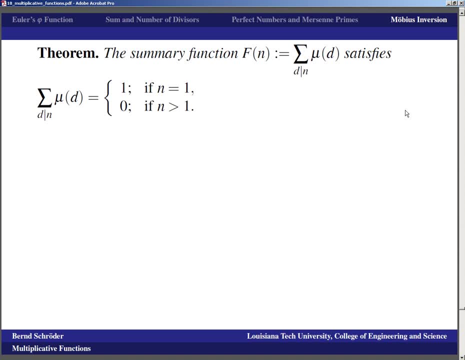 greater than one sober. basically just building up some facts about the new york's function, similar to what we've done for the order fee function is just one. it's just that for the order fee function we saw a little bit more motivation early on, and here's the proof. 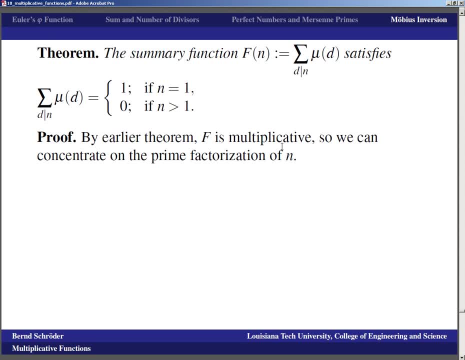 well, we've got an earlier theorem that says that the summary function is multiplicative, and so that means we can concentrate on that prime factorization often. so first note that for uh, an exponent k in a prime number p, we have the effort. p to the k is the some overall divisors of p to the k. new york t. 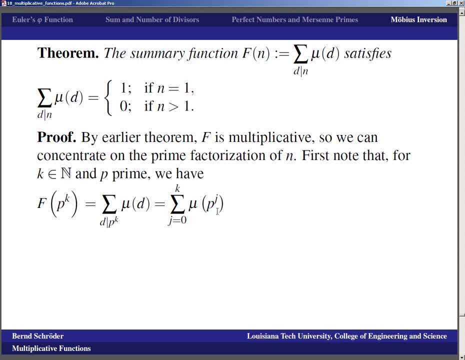 which is the some j equals zero, became you to the new york p to the j. and that's because new york one is one, it's negative one. because new york p is negative one to the first, plus the some j equals to became you will p to the j. 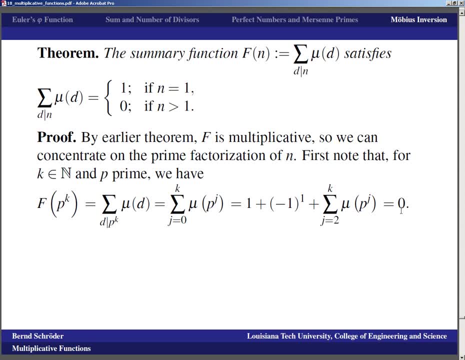 those guys are all zero, and month was minus one zero, so the whole thing is zero. and that means, if this is the prime factorization of the number greater than one, well then, if often it's if off this product, which is the product of the f of pj. 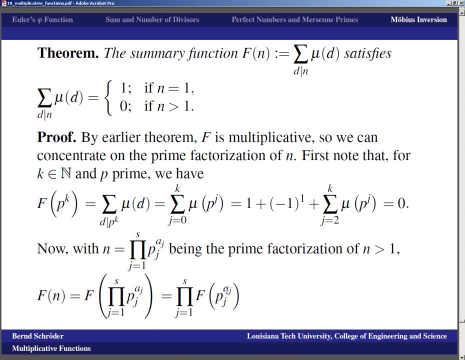 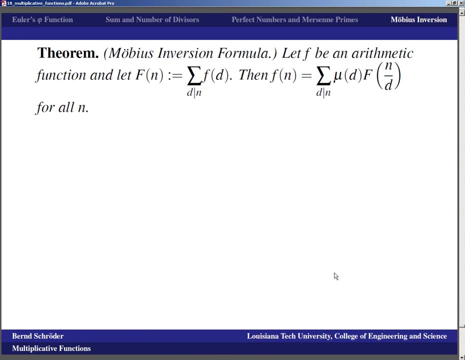 pj, pj, pj is equal to zero because, no matter what i do, these exponents are all non-negative integers. weekend the product of visa. all right on, now we are going to prove. the nueve is inversion factor. slides, i think, and that is if you have an arithmetic function. 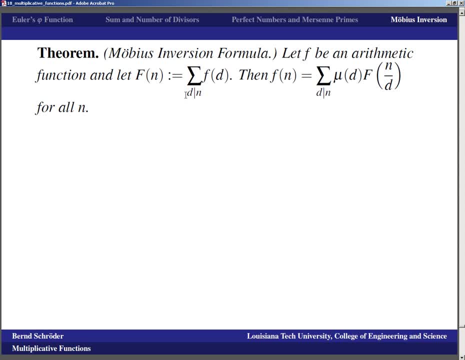 and off this arithmetic function- you know the summit of function to some- over all the d set divided in. if off t you can get the function box. if u summarize over all the d divides in, you off the info in over t and others. true for all national numbers. it. 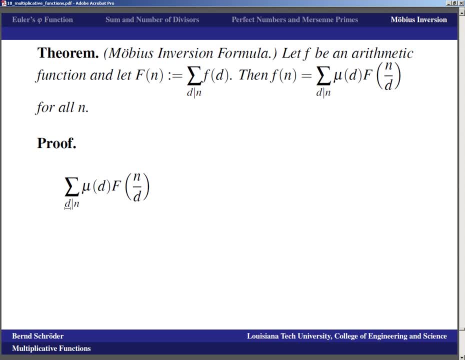 okay, so we just start on the right and see what happens. so this is some over all the fighters of in you off the info in over t, which is the some over all. do you over in you off the into uh times to some or overall either divide in over t. 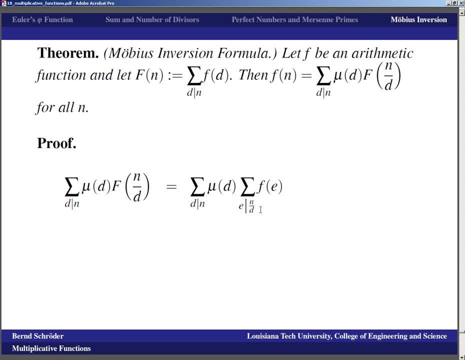 info fee. and that's just a definition of the summit of function. all right, now we can certainly pull this out and turn it into a double. some of you off t times, therefore e, but now we've realized he this is a somewhere we first specified advisor off in and then look at all the devices you've been over t. 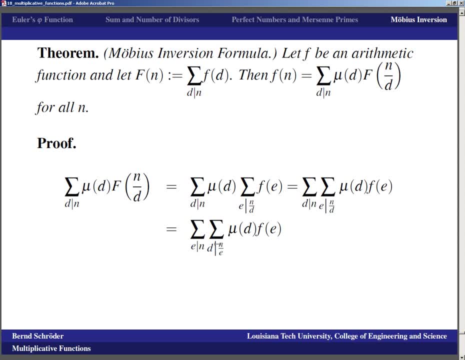 we could have equally well specified advisor you off in and then a divisor off in over e in. we would have ended up with the same product whether we choose the e first or the dee first. both summations run over the same sets pairs of numbers and that means that this is to some over all e divides in info fee times to some. 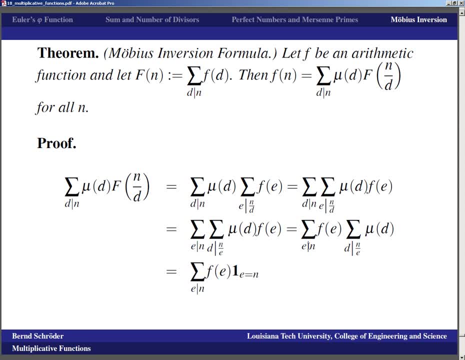 overall d divides in over e, you off t and what we know from that- and here's where i'm using uh notations- that is more familiar to people in probability theory we had just proved in the previous limit that this some is equal to one exactly when he is equal to in, because the sun is only equal to one. 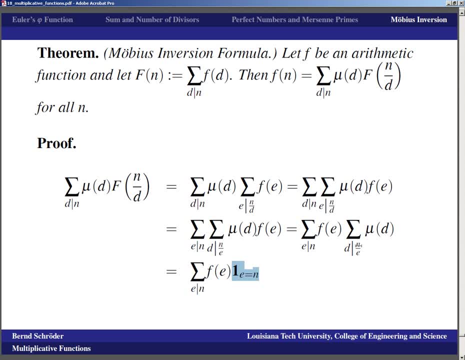 d is equal to one year and uh, for all greater keys, the some or this on this is equal to zero, undisputed. tying up my time here, this some is equal to zero. we can divide by he is not one and that means the sun is only. 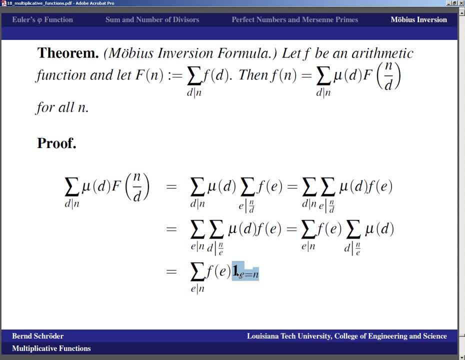 not non-zero when he is equal to end, and at that point it's exactly one, and so that means this is some over all. e divides in effort, e and the only summit that doesn't have a zero factor. easy equals, and, and so that means that we get it for in at the end. 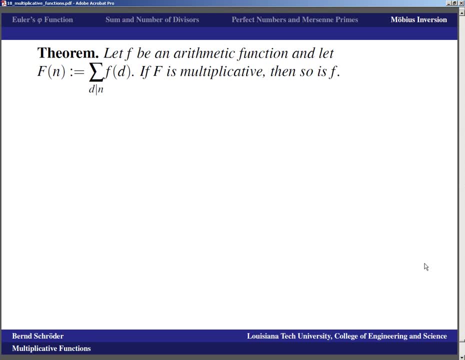 okay, and that should now give us that, if you have an arithmetic function, a, june eight, eight, if i think these, this summit function over all the fighters of in, if of d, if this summary summit function is market, then so is the function that we were something. so that is the converse of something. 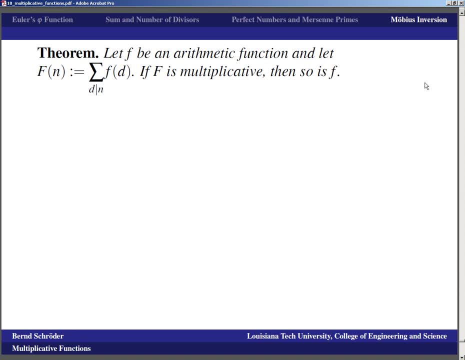 that we proved nearly in the field of the function section. well, to prove that, something a little big if we need to members him in that have. greatest comment on one if of in times in is from the previous fall formula. it's the sum overall divisors of in times in view of d. 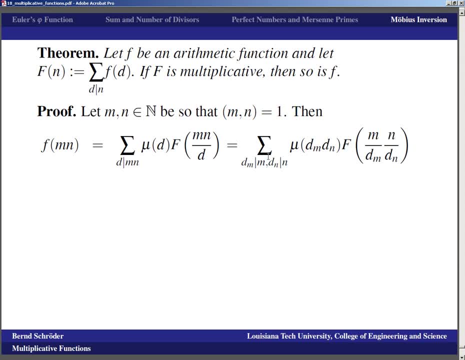 if of in in over deep ins are. that is the sum overall divisors of in in all the prices of in which we call d m and d? n new of d in d in if of in over d m in d in. so we're just letting that up. 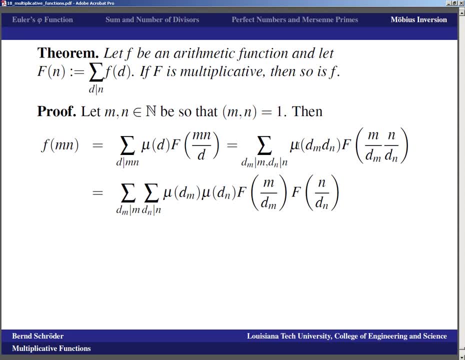 and now we use that as well as new or multiplicative. so this is still the sum over all the d m, c and the ins new of the in view of the in if, of in over d m, f, of in over d in, and for always using your, of course it. 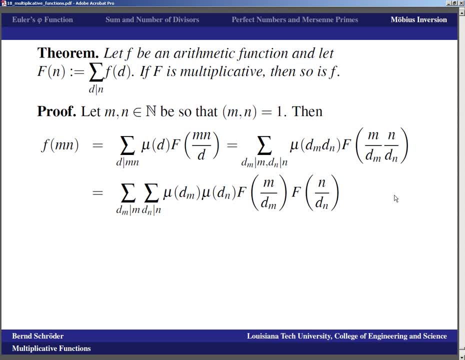 d m and d n, as well as these two fractions, have greatest common divisor, one, and now we can just factor stuff out. this is the sum overall: the d m divides in new of the in if of in over d m. d in divides in new of the in info. 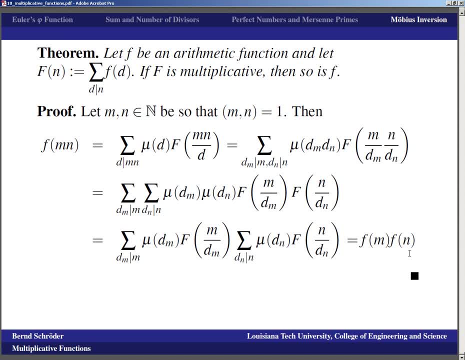 in over d in, and that's if of in times, if of in, and that is the in off this. okay, i jumped over it a little bit quickly and, to be perfectly honest, that is because i was very happy to cut through the proof of the new views inversion formula. 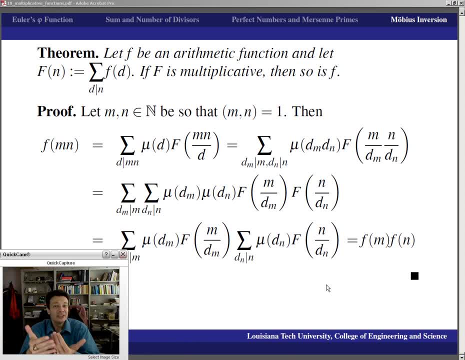 if you analyze the proof of the new views inversion formula, you basically see if you want to get a formula that expresses the function lower case f in terms of the summit of the function capital f, then that computation, if you just throw in an arbitrary factor, you there that competition shows. 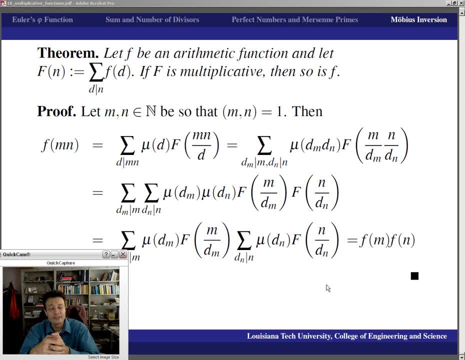 the properties, that the function you would have to have and that probably, hopefully, uh, or if not, then he had some other brilliant idea, but uh, that is the kind of thing that can be mathematicians: to define auxiliary functions such as the new view for maybe it's function.